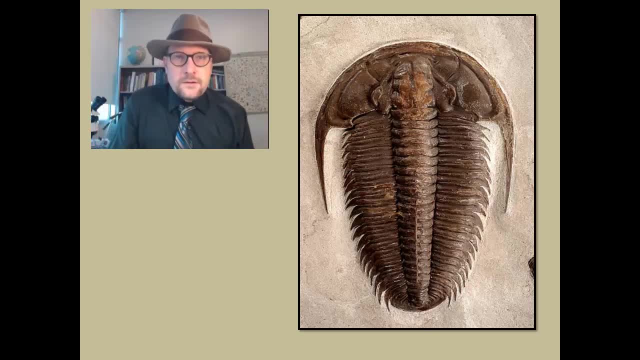 and principally focus on the famous trilobites. Trilobites, despite being extinct for over 250 million years, are still fairly well recognized, even by novice paleontologists. There are exclusively marine organisms being found in many marine species and they can be found in many marine species. They can be found in many marine. species and they can be found in many marine species. They can be found in many marine species and they can be found in many marine species. They can be found in many marine shales from the Paleozoic era and they are placed within the larger group, the arthropods. 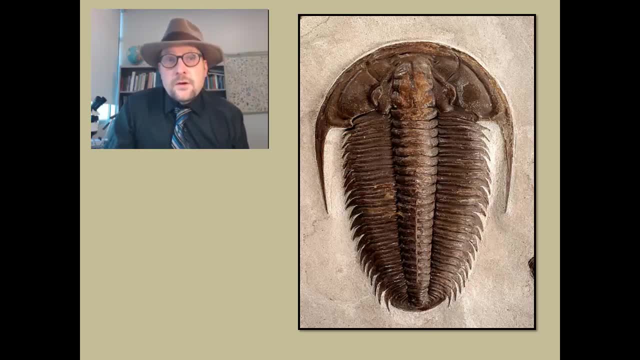 based on a number of shared derived features. These include a segmented body, a character shared with annelid worms and appears to be a protozoom character. They all have paired limbs to each body segment. This is the first group we have looked at that has these paired appendages. 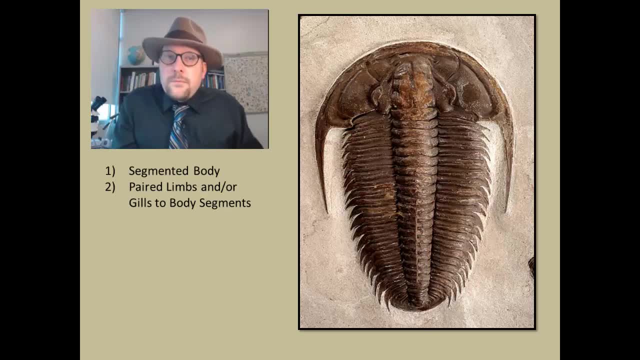 This is the first group we have looked at that has these paired appendages. Most of the groups are mobile, although some, like barnacles, become sessile. They have an exoskeleton that is shed. This is made of cuticle, chitin or calcium carbonate. 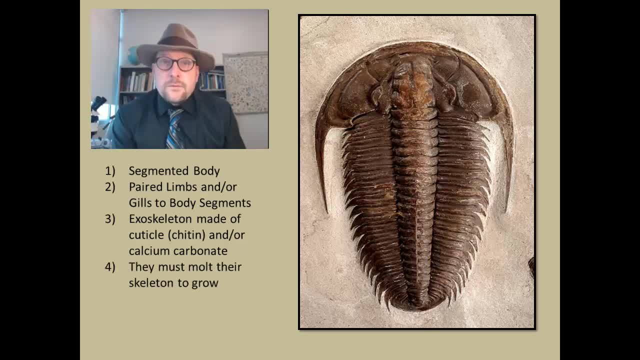 They have an external skeleton. They must molt their exoskeleton to grow. This means that many groups undergo morphological change with each shed of the exoskeleton And many groups undergo radical metamorphism, such as caterpillars to butterflies. Fifth, the final character of arthropods is that they have sense organs. They have things like 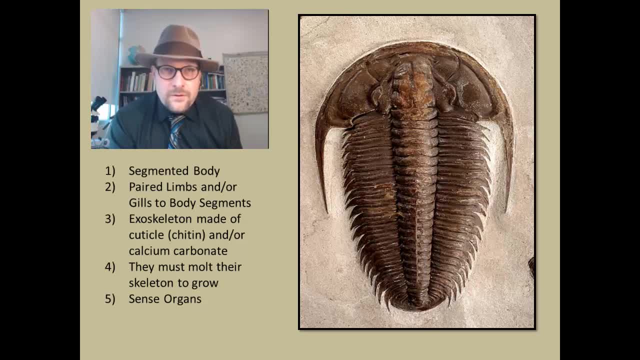 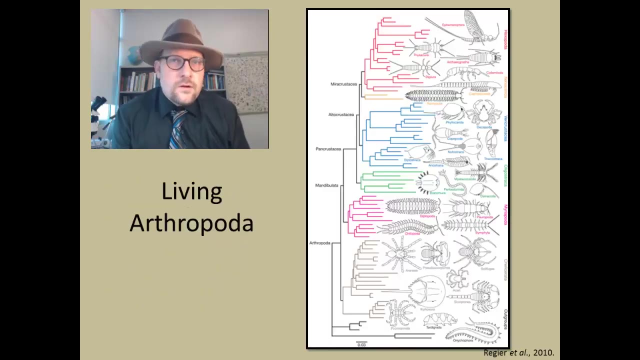 eyes and even have a small brain and nerve fibers that run through a central nervous system. The first group we have has very complicated sense organs. All of these characters are found within all arthropods. Let's take a look at modern living members of arthropods and see how they have been classified. 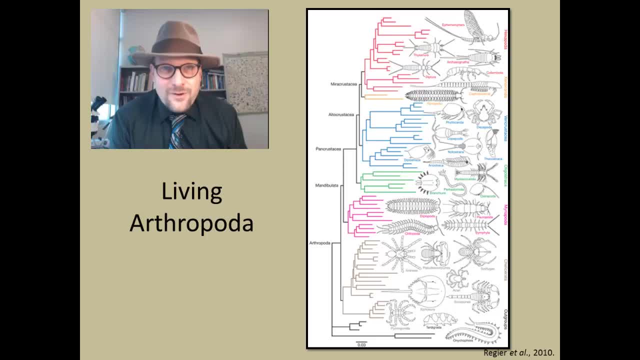 in order to see where we can try to fit in the extinct trilobites. Modern arthropods are broken down into a number of nested groups, each of which are extremely diverse and abundant. today, Most of these groups are terrestrial, though many of them are marine as well. 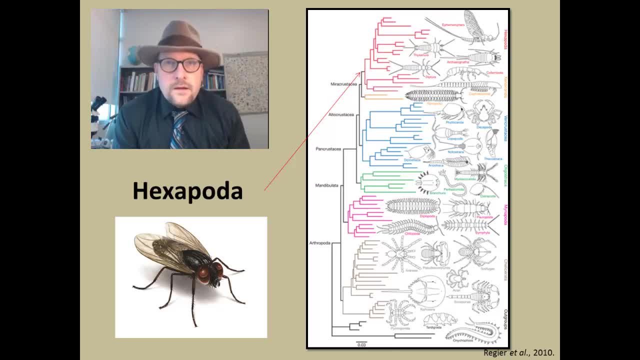 The first group is the most diverse: the hexapodia. These are animals that have six legs. They include true insects and flies, moths and butterflies and ants as well. Members of this group are extremely diverse, but they all have the same basic body plan. 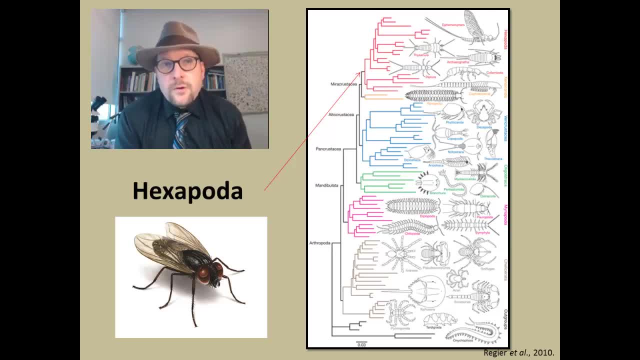 They have an anterior head, a thorax and a posterior abdomen, with three paired legs. So trilobites with their many legs and segments are not a member of this group. The fossil record of arthropods is that they have six legs. 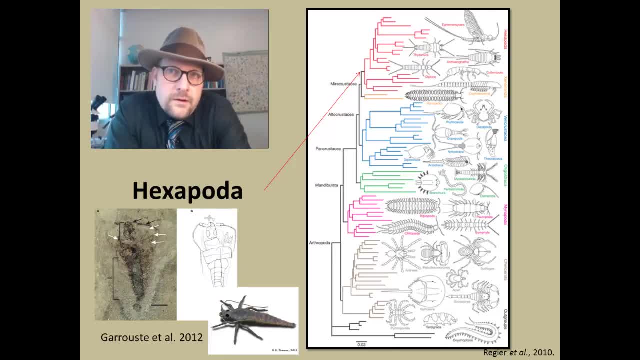 They have three pairs of legs and a segment of body with a head, thorax and a larger abdomen. These early Devonian insects are close to appearance to modern springtails, which belong to a group called the endognathia. The endognathia basically means that the mouthparts are retractable. 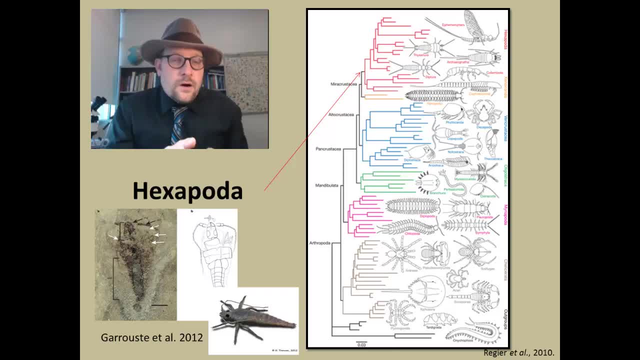 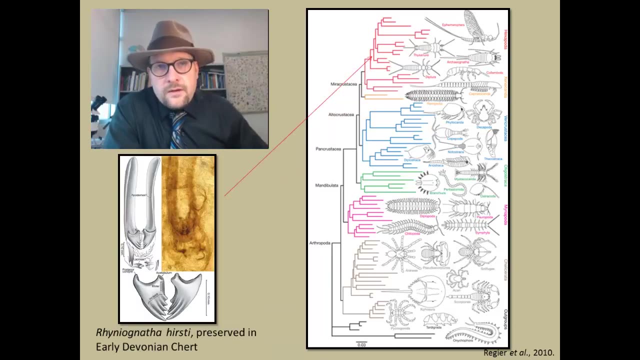 They have a very large mouth. They are attracted inside the head. This group includes mostly wingless insects such as springtails and other bugs that you find feeding on decaying matter on land. The other major group of the hexapodia are the ectognathids. 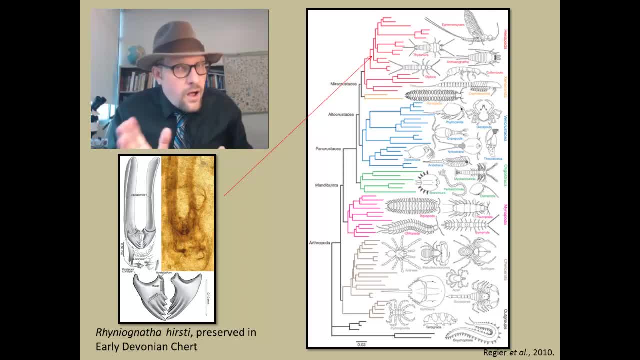 These mean that the mouthparts are outside of the head. They also have a fossil record that extends all the way back to the Devonian. This group includes many winged insects. This seems to be some evidence that the origin of flight in insects originated sometime. 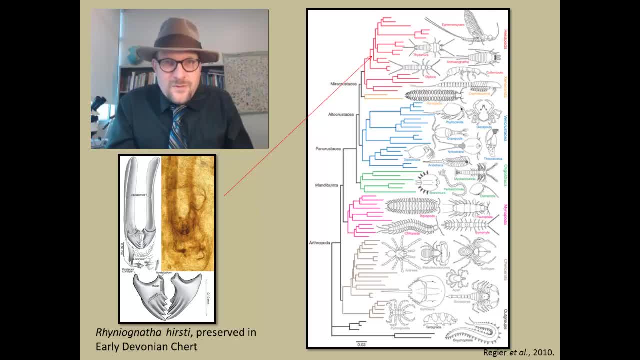 during the Devonian, or maybe even earlier. just as our ancestors were starting to learn how to crawl out onto land, so insects had us beat by a long shot in terms of colonizing land and developing the ability to fly, going all the way back to the Devonian. 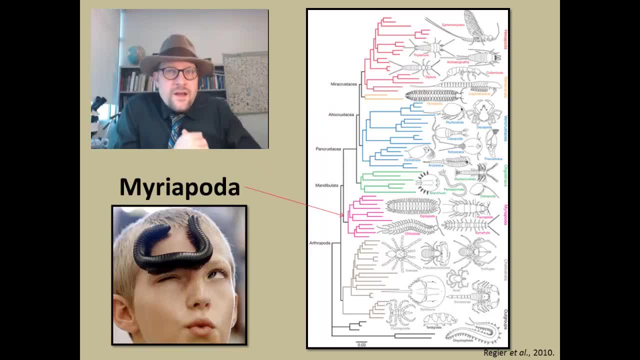 The hexapodia are often regarded as a sister group to another major terrestrial group, the myapodia. The myapodia include centipedes, millipedes, and, as you can guess from their names, they have many legs rather than being restricted to just six legs. 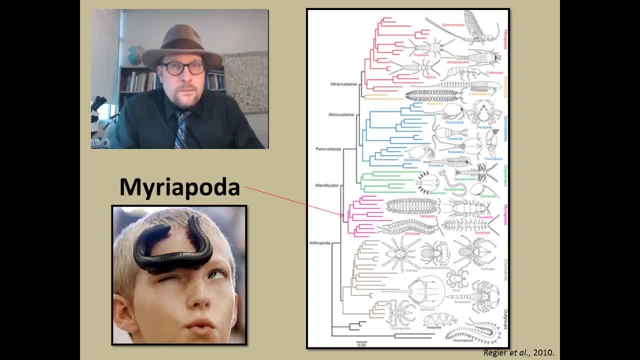 The myapodia have been removed as a sister group to the hexapodia, based on molecular phylogenies that place the crustacea as more closely related to the hexapodia. This phylogeny indicates that the hexapodia and myapodia independently relate to the myapodia. 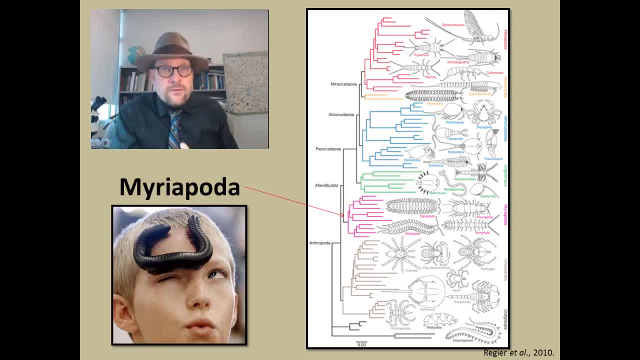 The myapodia is a sister group to the hexapodia. The hexapodia is a sister group to the hexapodia. The hexapodia and myapodia came out of the water during the Paleozoic to diversify on land, and so you have two groups that come out of the waters and become specialized to. 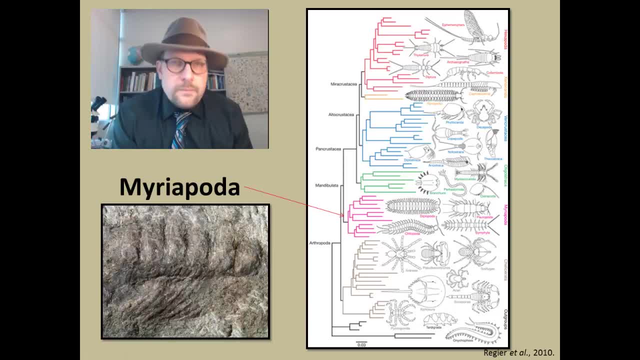 living on land. The fossil record of the myapodia goes all the way back to the Silurian, indicating that the myapodia have been one of the first groups of animals and plants to become land living and the first animal to develop a respiration system. 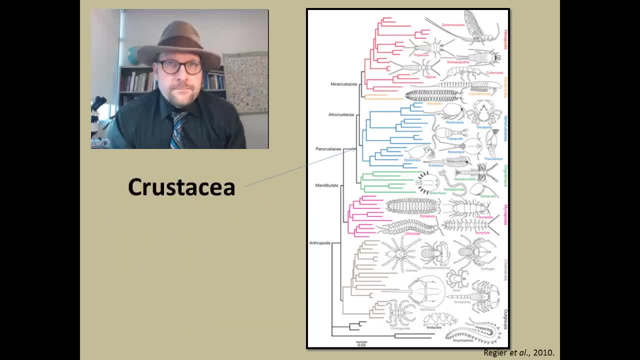 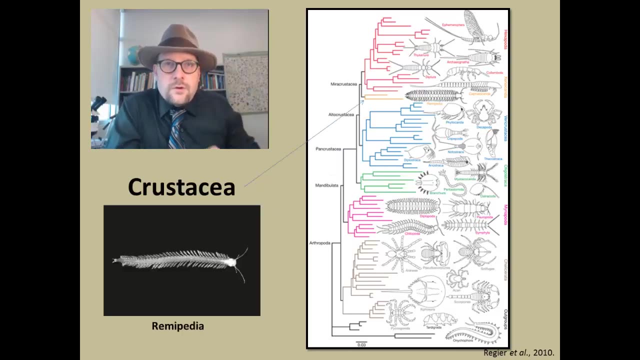 Now between the myapodia and the hexapodia, is a really diverse group of aquatic organisms, the crustacea. These include things like the branchiopoda, the brine shrimp, and a really weird group called the remnopoidae. 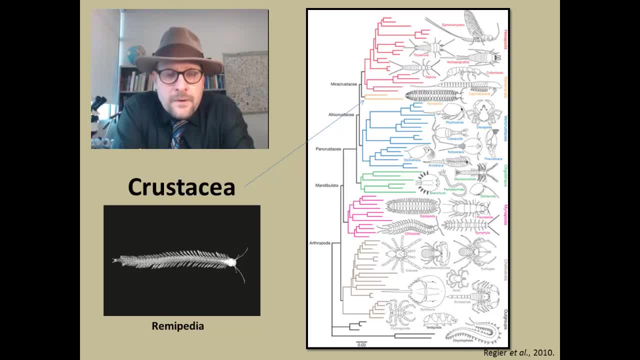 These are blind crustaceans that look like centipedes that live under water. Many of them are blind and live in caves. They have a lot of fun. They have a lot of fun. Their phylogeny is they fall out as a sister group to the hexapodia, which is interesting. 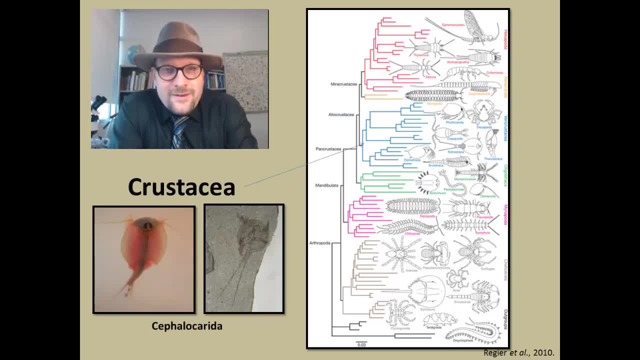 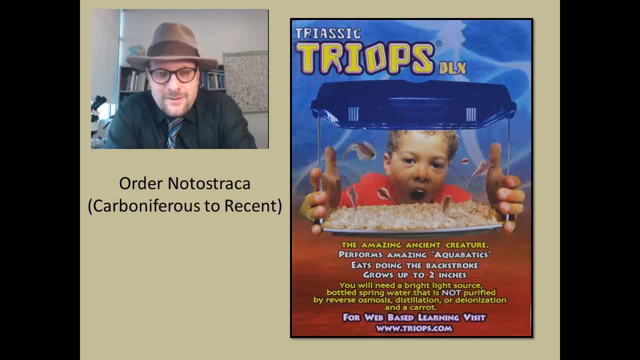 There is also the cephalocardae. These are the horseshoe shrimp, but you probably know these as triops. These are the famous group of little shrimpers that people take home as pets from hobby stores and stuff and they take their eggs and they hydrate them and they hatch and you get these. 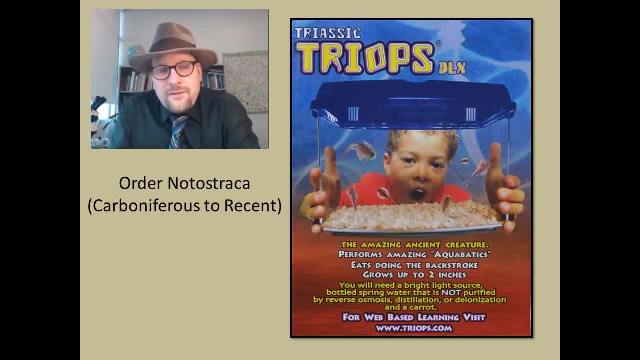 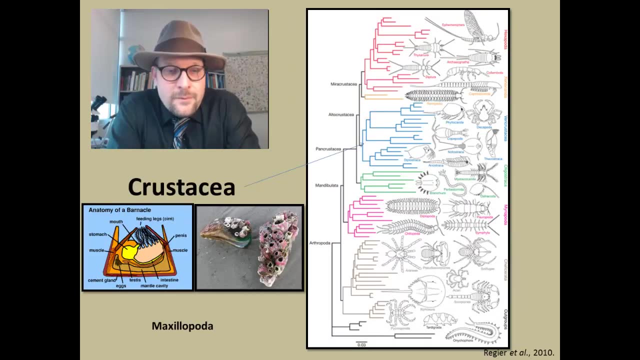 little triops. Now, these are an interesting group because they have a very extensive fossil record, going all the way back to the carboniferous, so they are an example of a living fossil. The next group are the maxiopodae. These include the barnacles and fish lice and some other things. 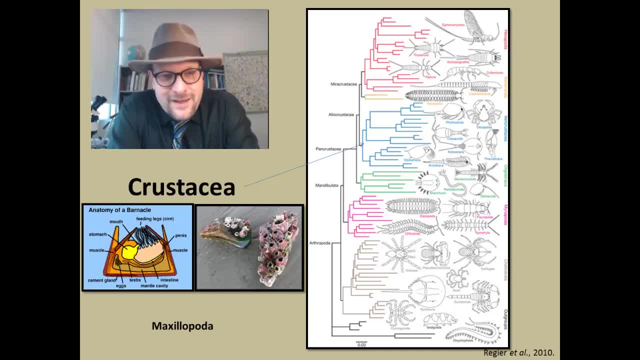 Barnacles are just bizarre creatures. They are an arthropod that decided to become sessile, So these are related to shrimp. They develop an exoskeleton that they can continually grow and live with. They can live with their family. They can live with their friends. 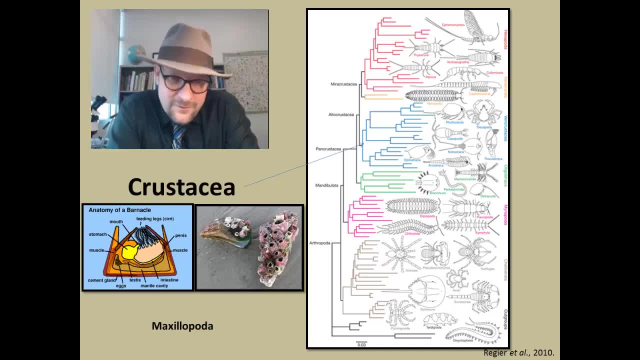 They can live within a sessile sort of form, living burrowed against organisms. Here's some on some bivalves- You see them on ships and stuff- and they basically will throw out their feeding legs. These are actually their legs that they throw out and bring in food into their mouth and 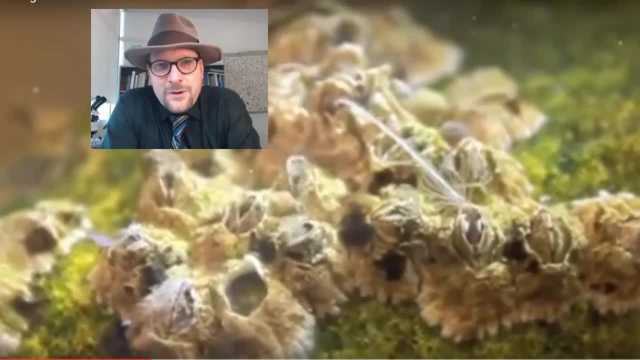 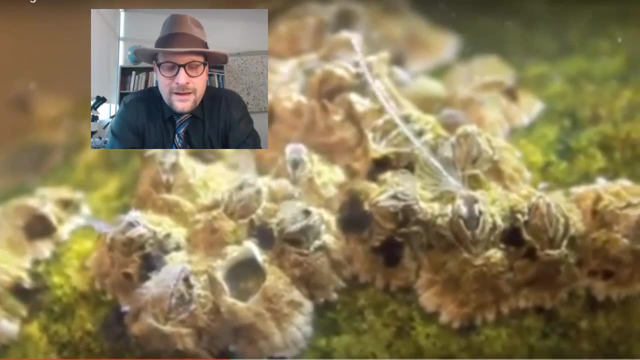 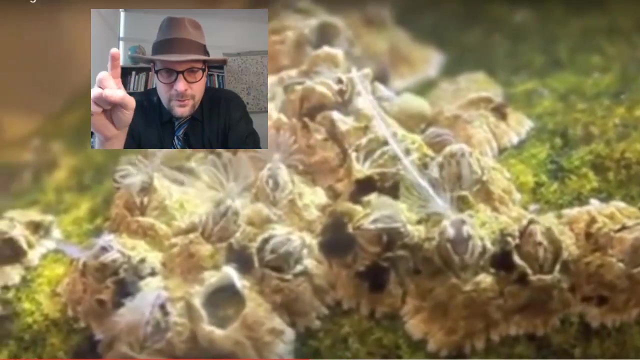 they're just really bizarre and unusual creatures. I just want to show you a quick video here of some barnacles. You can see they're throwing their little legs out. These guys are actually mating, So that long strand is a penis that is extending out of the barnacles and going in and prodding. 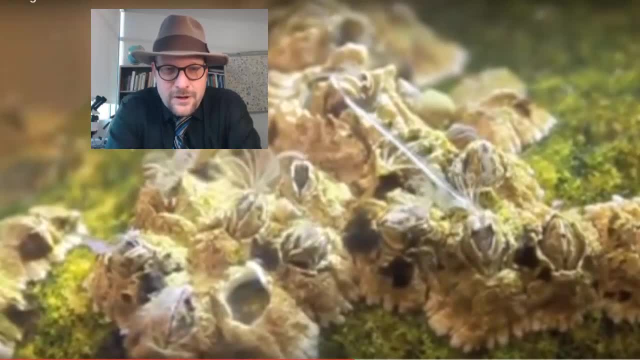 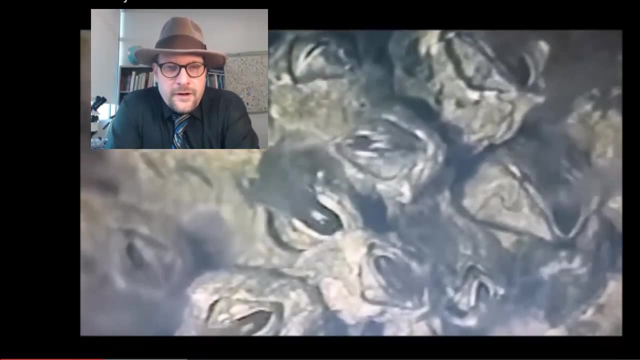 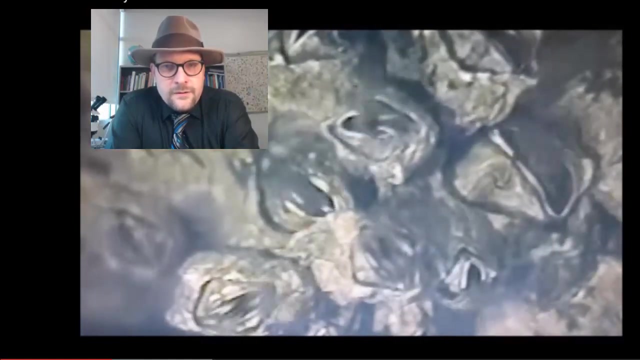 various other members of the colony for sexual reproduction, to deliver the sperm to each one of those individuals. This video here shows some barnacles that are actually feeding, and you can see how they're using their feet to sweep the water and catch food and bring it down into their little shelled. 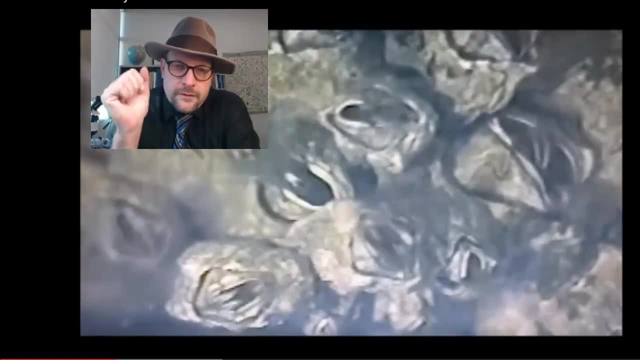 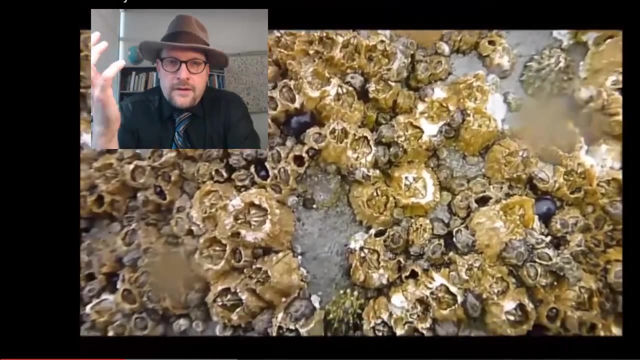 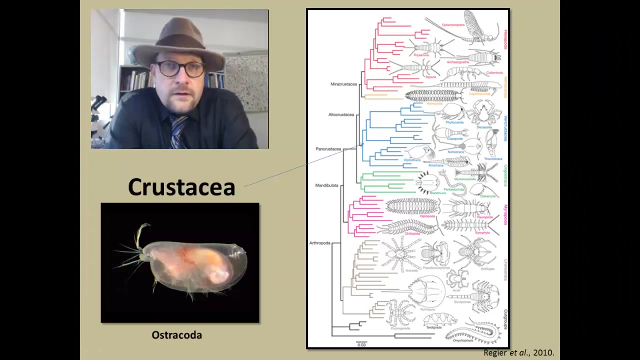 structures there, So they send out their feet. like this: Their little mouth is grabbing hold of things as they're feeding. This is an example of an arthropod that has become a sessile organism. The next group that we have in here are the ostracoda. 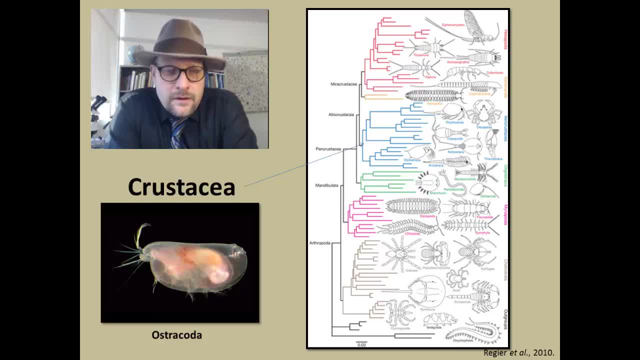 These are sometimes referred to as seed shrimp. The ostracoda have a fabulous fossil record and they make it into freshwater systems. The ostracoda are basically shelled shrimp. That's what they are. They have a hard calcium carbonate shell that they produce on either side of them to help. 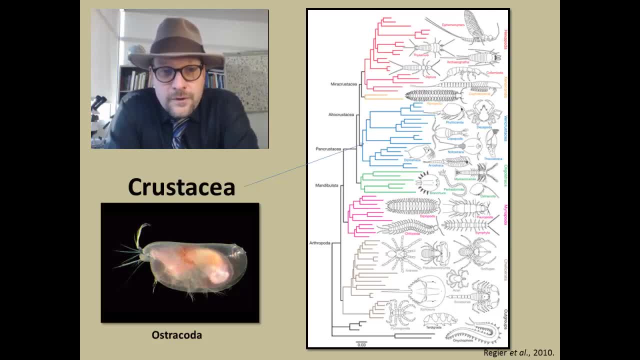 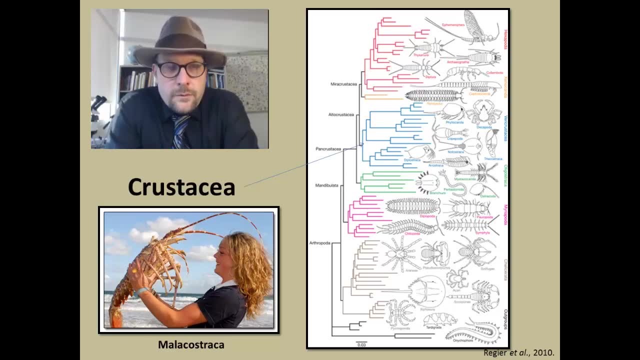 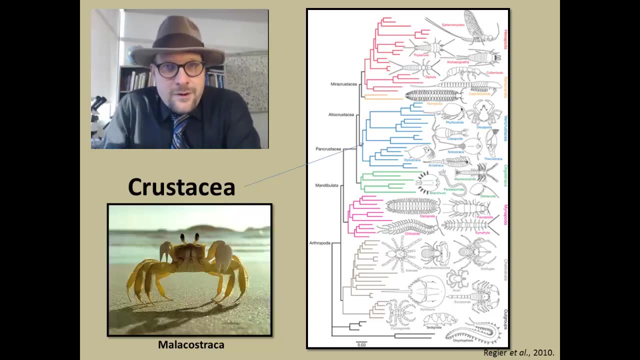 protect them. They swim around, often times in huge numbers, feeding on various detritus in the water. The last group is the group you're probably most familiar with. These are the malacostria. These include the lobsters. they also include the crabs. 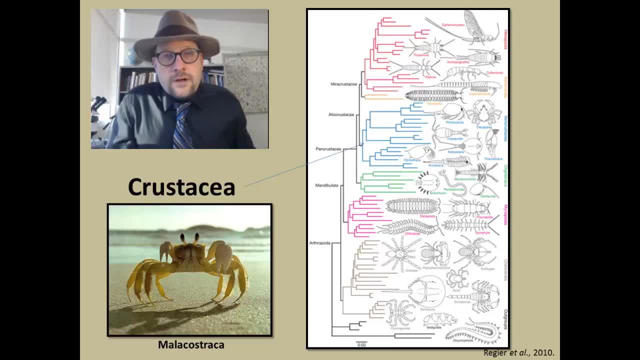 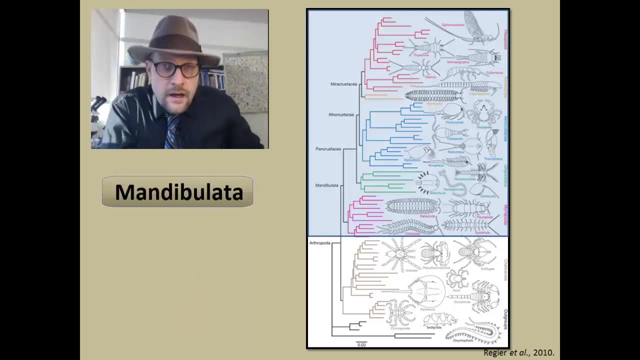 A lot of shrimp are in this group as well. So those are the crustacea, These are the ostracoda, And those are now kind of regarded as the sister group of the hexapodia, which is kind of interesting. Now, together the hexapodia, the crustacean and the myropodia form a clade and this is 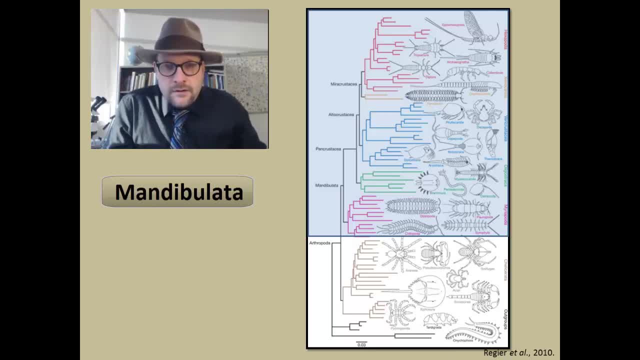 called a mandibulata. Now, mandibulata is a very large group of the arthropods, so this includes all the millipedes and centipedes and all the crustaceans, the shrimp, the lobsters, the barnacles, the little. 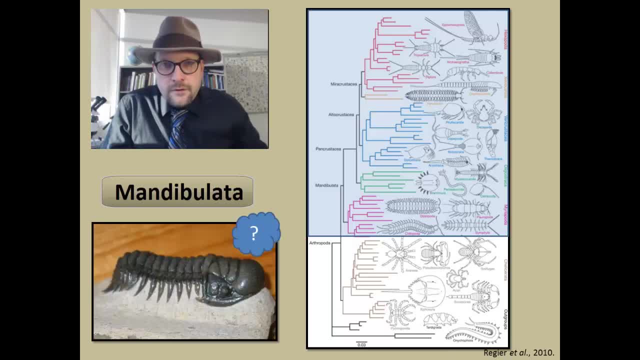 lice, shrimp, and includes all the insects as well, So a pretty diverse group. So one of the questions we have with trilobites is: are they members of the malleopoda? So this is one of the interesting questions we can ask. 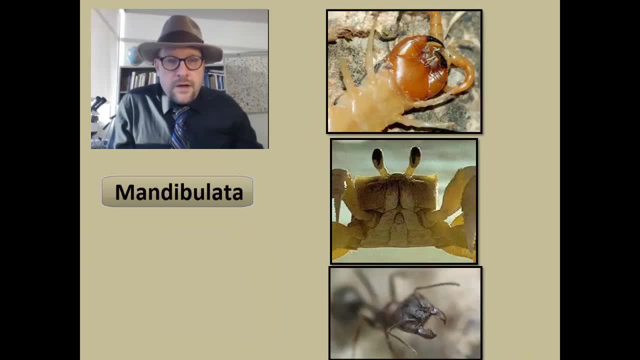 So now the malleopoda are held together by the fact that they actually have a mandible, So they possess a paired mandible apparatus. And now this apparatus is different than what we'll see in other groups because it's used in food gathering and chewing. 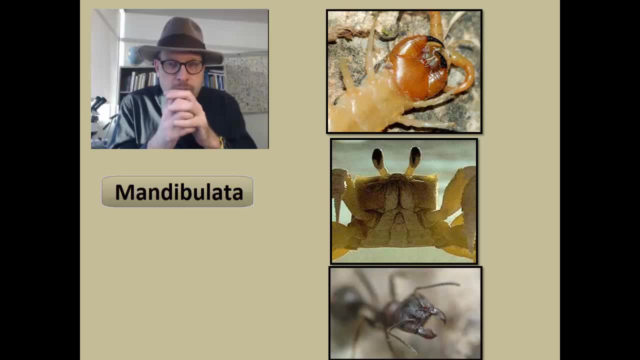 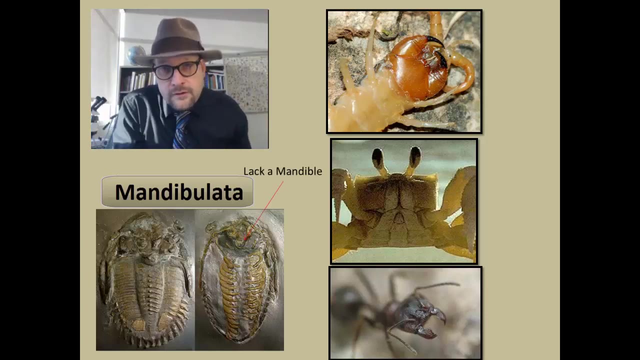 So it's actually used to grab hold of food And they actually bring it in and actually masticate or break up the food into their mouths. So these groups are all united in having a mandible sort apparatus. So if we look at specimens of trilobites that actually preserve the ventral parts of the 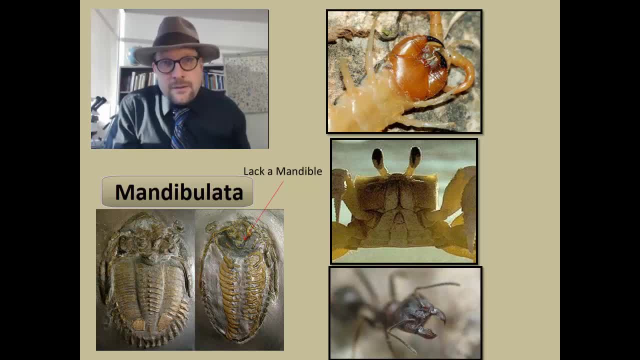 surface of these guys- the mouth, the mandible, the malleopoda- actually lacks any paired mandibular apparatuses And so, as a more primitive configuration- That's this- There's no specific group for the mandibleapec. 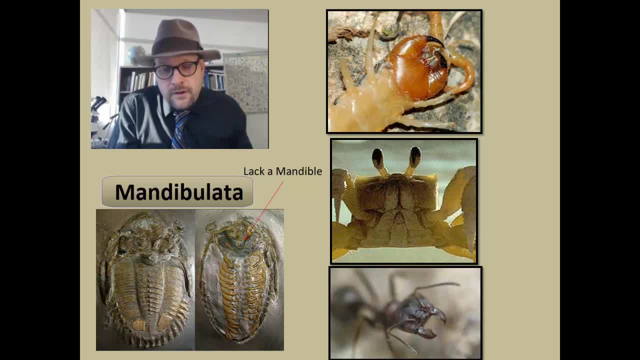 place the trilobites between some of the more primitive members of the arthropod groups. So let's take a look at what some of these strange creatures that are more primitive within the arthropod giant, huge bushy tree. The first group is the Cherocetria. 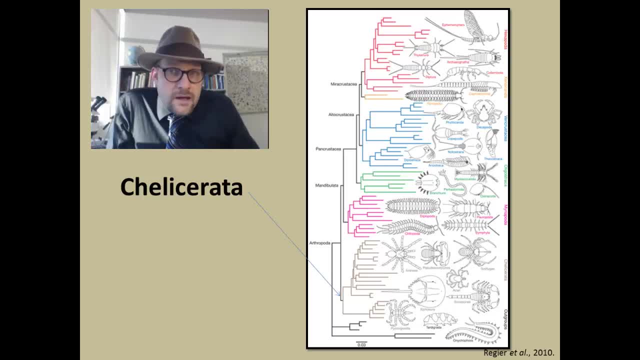 These include a very diverse group of arthropods that many authors suggest form a monophyletic group. They are united in possessing a serrate area, a paired appendage that can carry food into the mouth. So it is kind of like some claws have pinchers that can grab hold of food and put it in the 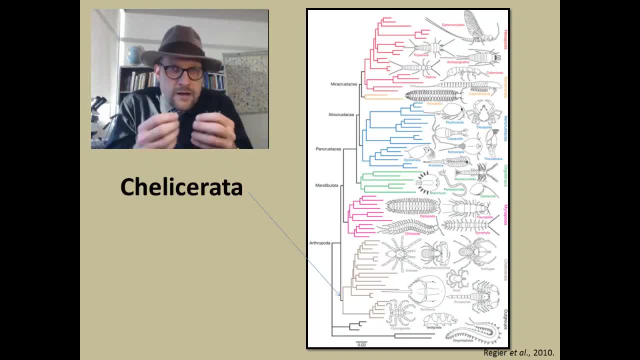 mouth, but it is not used in chewing or any sort of mastication. Not all groups have a cherrata, and some crustaceans utilize claws in a similar manner. Another defining feature of the cherrata is the fact that none of its members exhibit antennae. 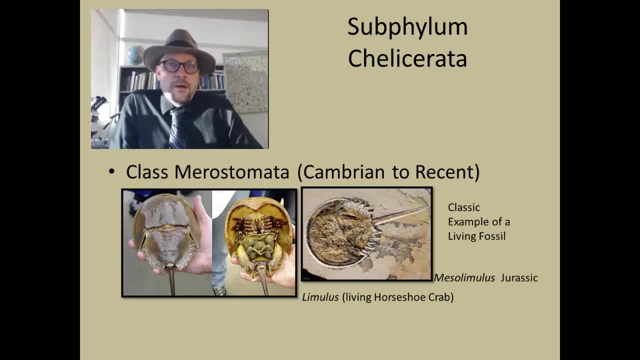 The cherracerata include the meristoma, which includes the modern day horseshoe crabs, litimus. Fossils that closely resemble litimus extend into the fossil record going all the way back to the Mesozoic. The genus Mesolimus from the Jurassic of Germany closely resembles litimus. 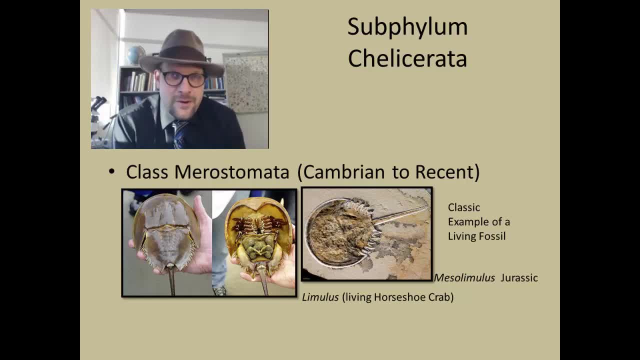 It looks exactly like a modern day horseshoe crab. This makes the genus Limnus a good example of a living fossil, where, for long periods of geological time, the morphology of a species does not change significantly. The meristoma has a fossil record that extends all the way back to the Cambrian and, unlike 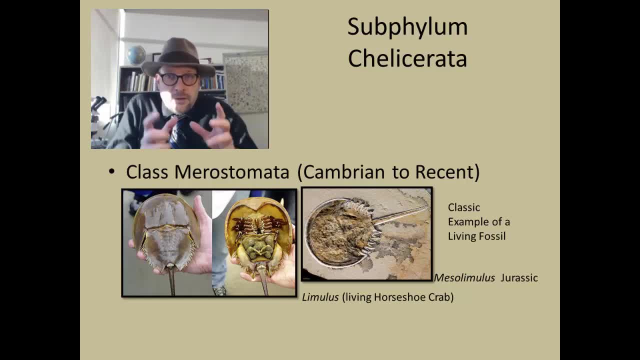 crabs and lobsters, members of the meristoma, don't have those mandibular appendages or teeth like jaws beside the mouth. Instead they have a set of pincer-like appendages at the front of the mouth for grabbing food. 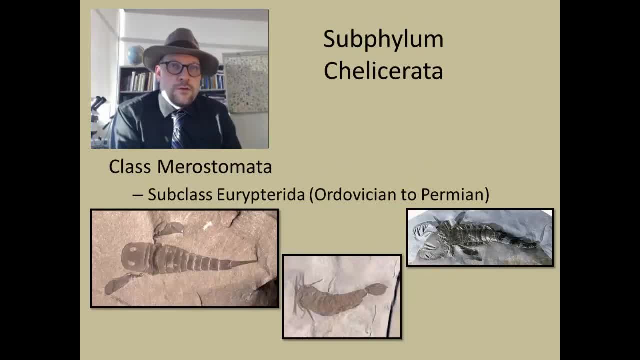 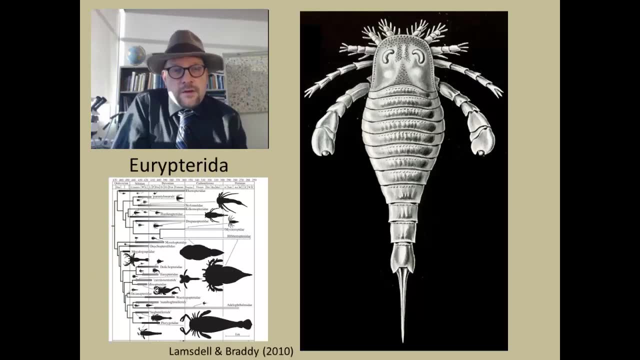 but are not used for chewing. Closer related to the horseshoe crabs, often times placed within the same class, is the sea scorpions, the Euryopterids. The Euryopterids lived from the Ordovician to the Permian. having fallen victim to the 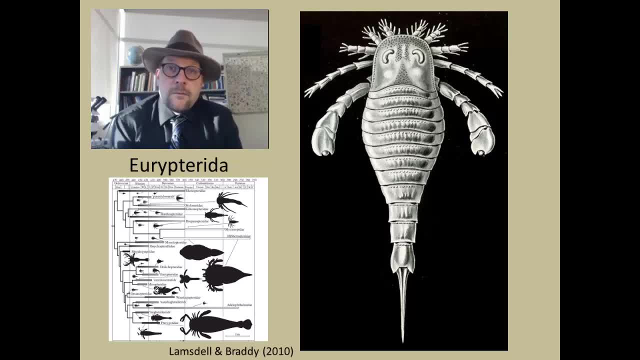 Permian-Triassic extinction. just about like everything else, Most members of the Euryapsids are rather small, But some forms got to be really big, about 2 meters in length or so. They likely lived on the ocean floor sculling around, and trace fossils have been found. 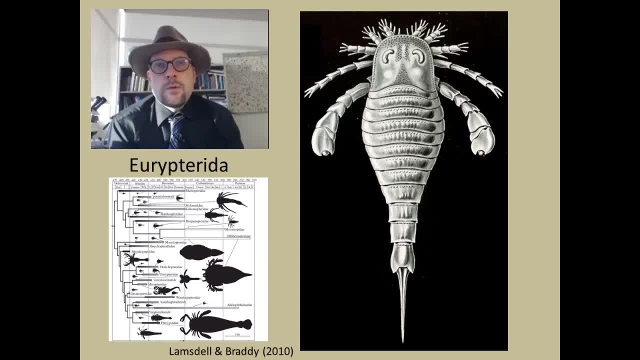 to indicate that they could crawl along the surface. Some people have even proposed that they were able to come out of the water for short periods of time. They are most diverse during the Silurian and, with the first occurrence of their fossil record during the Ordovician. 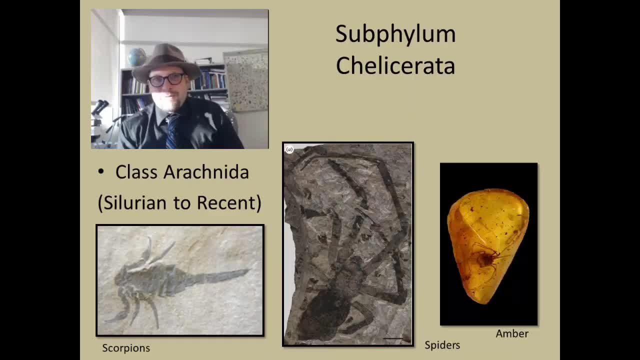 The next group of the Cheria serrata are the very diverse. The Arachnids, which include spiders and scorpions, are another group of arthropods that become specialized for life on land. This group has a fossil record that extends all the way back to the Silurian. 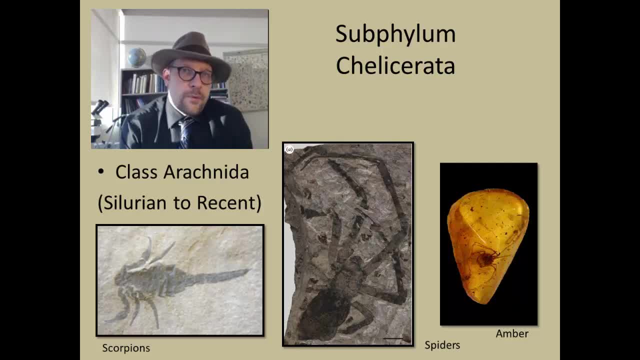 In fact, the Arachnids are likely the first group of arthropods to diversify for life on land and probably co-occurred with those early land myopodia. The group has a really good fossil record, Despite the fact that their exoskeleton is made out of chitin they don't preserve. 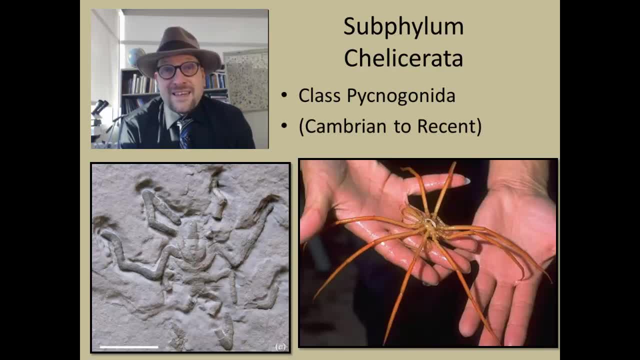 as well. The last group of the Cheria serrata are the sea spiders. This is one of my favorite groups. These are a fully marine group of arthropods living on the ocean floor. They have a great fossil record going all the way back to the Cambrian. 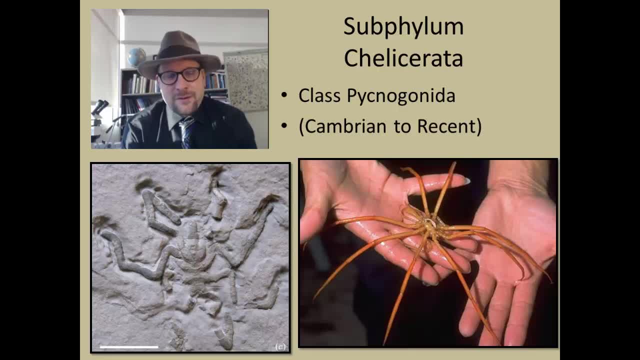 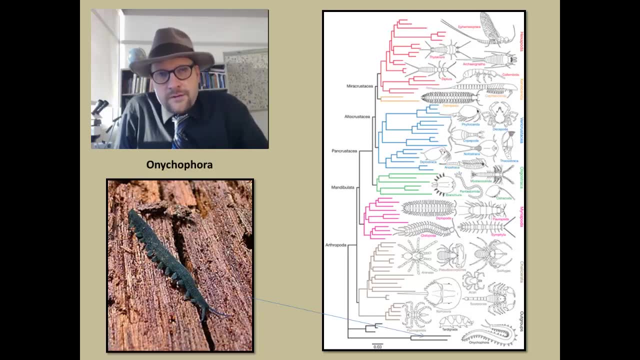 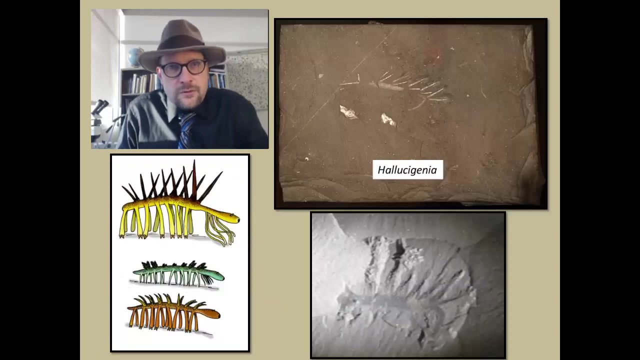 Very bizarre group and just very weird. There are two other groups that are found, often placed as outgroups. The first group is the Velvet Worms. these are the Onchleophoria, which mean the claw bearers. They are often to be related to the very strange and bizarre Haliginthia from the Burgess Shale. 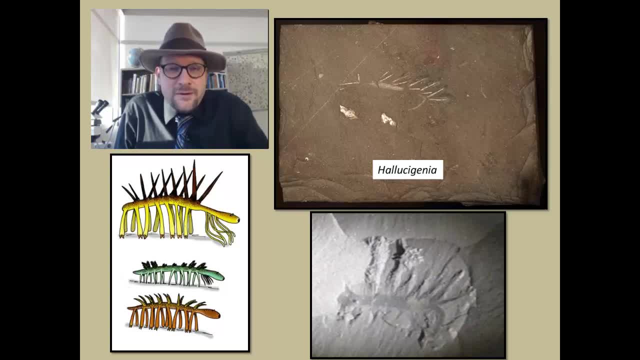 of Canada. These are weird fossils that people have puzzled over what they actually are, but most people place them within the Velvet Worm group, the Onchleophoria. They have segmented spines or limbs that project out of the skeleton, so they are often placed. 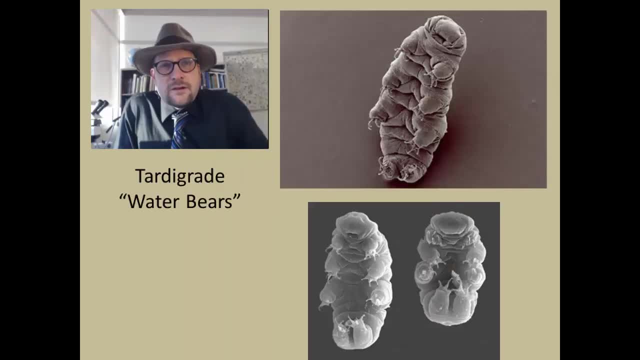 outside of the arthropods. The next group that is often entered into discussions of arthropods are the Ptolegaids, or the water bears. These are really teeny, tiny like worms. they are segmented bodies, super tiny, very microscopic. 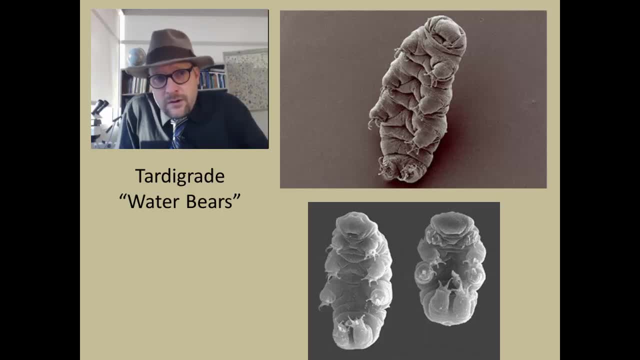 little organisms. Recent studies have suggested that the tardigrades are maybe possibly more closely related to nematode worms, and that is based on some of the molecular data that is coming out. Some studies have suggested a possible relation to arthropods, including some of the things: 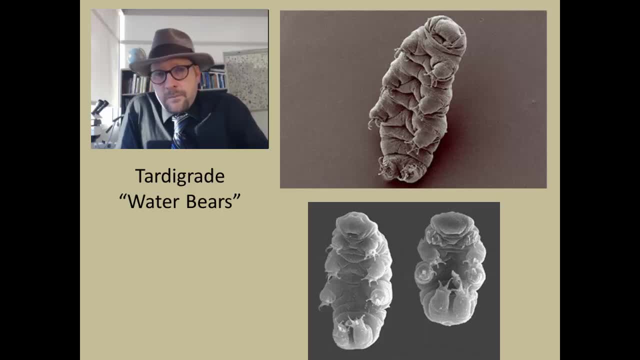 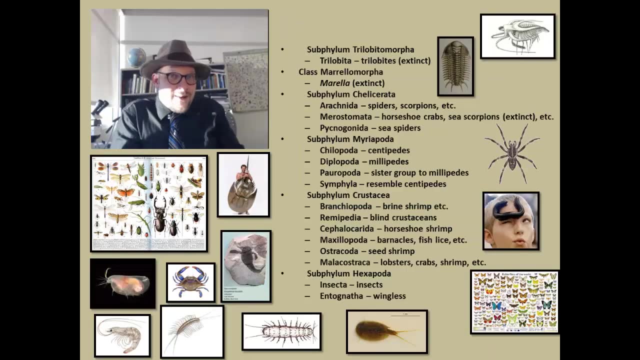 like dust mites and some of these really teeny arthropods We will have to see. Here is the list of the massive nomenclature of various arthropod groups and this is based on what is presented in the textbook. The systematic position of trilobites is kind of debated as they appear to be closely related. 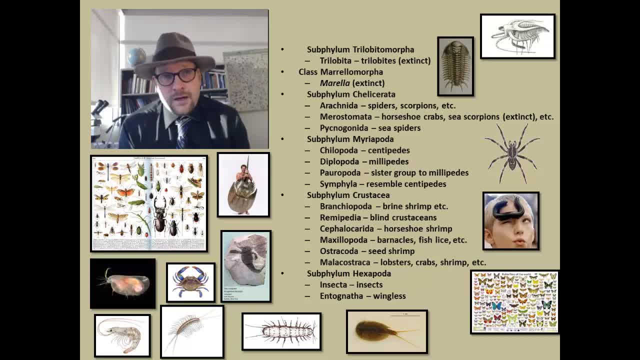 to both the Myrostomia and the Myopoda. This is a group of arthropods that are more likely to be related to both the Myopoda and the Maristomia. This is a group of arthropods that are more likely to be related to both the Maristomia. 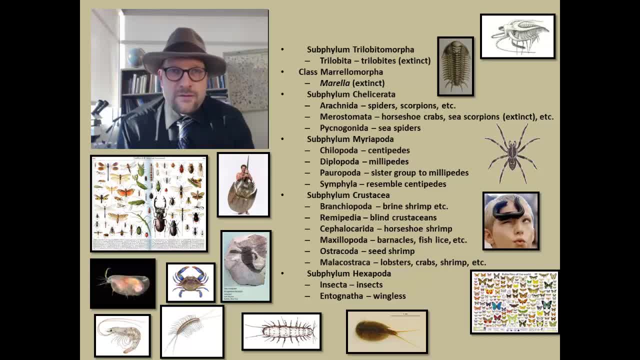 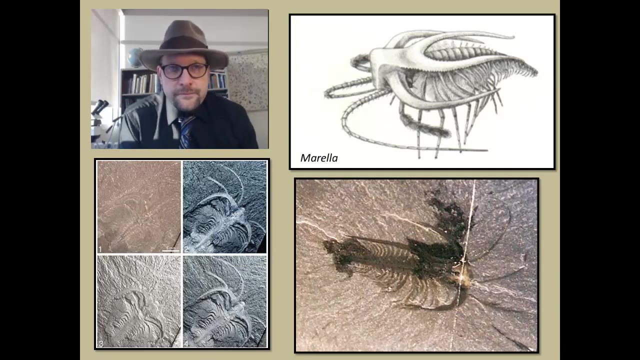 and the Myopoda. There is one fossil that seems to offer some sorts of Yar of the بعد Page. The Maristomia Maranea is the basis of the Maristomia. You'll probably be familiar with that. 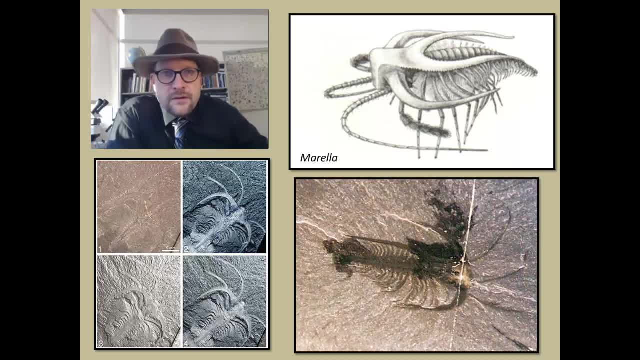 fossil site in British Columbia, Canada. It possesses a head shield with two large spines. anterior to the head shield is another pair of spines which project out to the side, and anterior to that is another set that extends the length of the body. 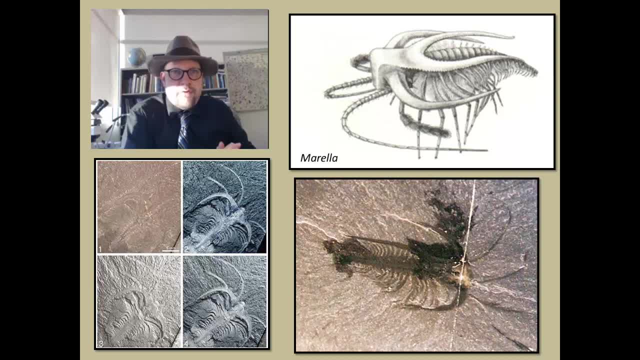 There are many body segments in which the appendages are feathery filaments or gills that were used during respiration. Marinara has a pair of rearward spines and a pair of antennae connected to the head shield, which means it is not necessarily regarded as a member of the Cercerata because those 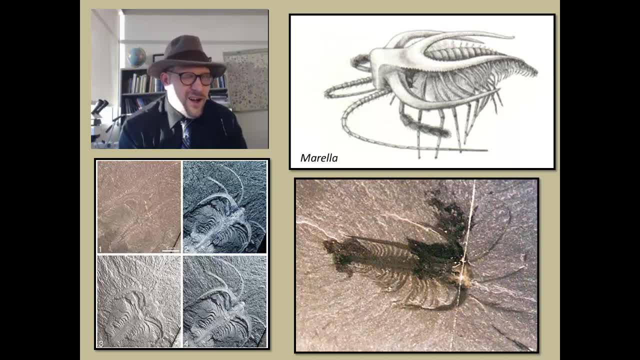 guys don't have antennae. However, trilobites also have antennae, so Marinara makes a good ancestral form for trilobites. Each appendage has two branches. The top branch is the gill used during respiration. The bottom branch is a leg. 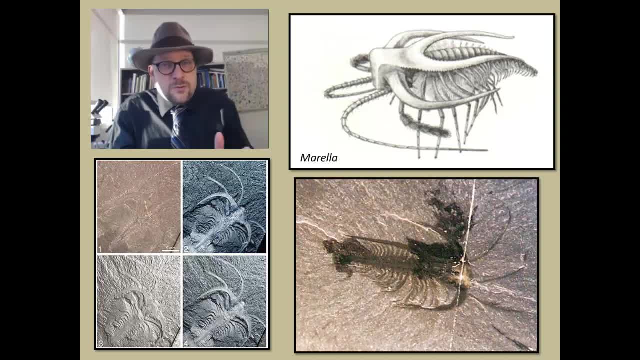 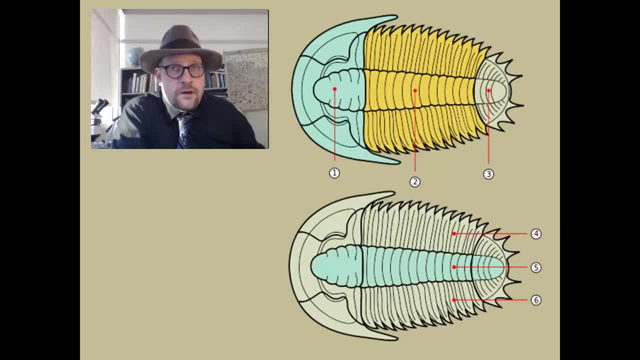 This is very similar to what we see in trilobites. As such, Marinara is often invoked as a stem trilobite. Alright, so trilobites are positioned within arthropods, possibly along with the Cercerata clade and the Myopoda clade. 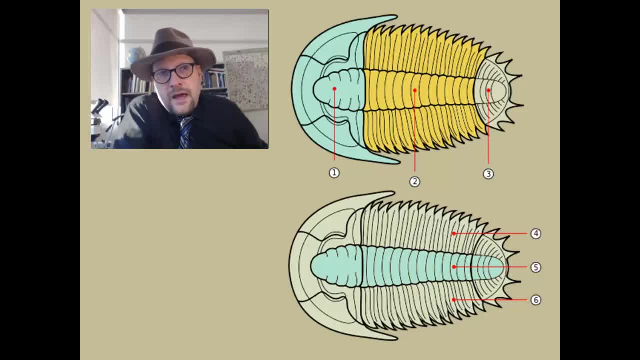 Since they both appear so early in the fossil record, they are often viewed as an early arthropod offshoot. that becomes very successful. during the Paleozoic, about 5,000 genera of trilobites known, so they are very diverse. 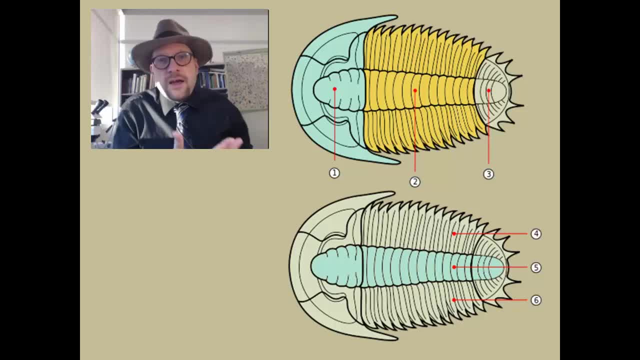 Let's look at some of the anatomical features of trilobites and define some useful terms. The trilobite body is divided into three major sections. it has the cephalon, the thorax and the pitigeum, which is the butt of the trilobites. 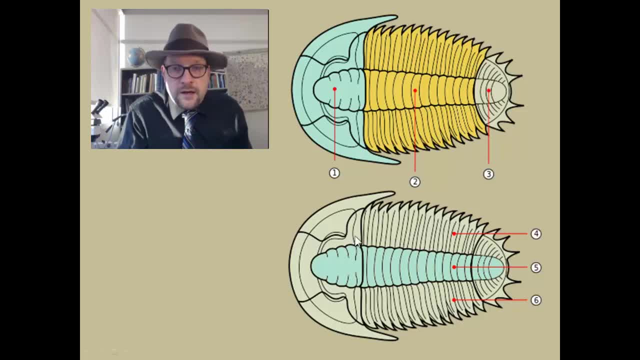 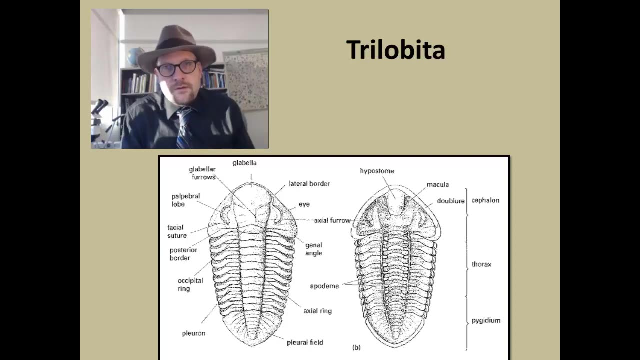 Trilobites are also known for having these three longitudinal lobes right, so its got a right and left pleural lobe and its got what's called the axial lobe, which is this part here shaded in blue. The cephalon, or head, contains the gabbliale, a raised protuberance on the center of the. 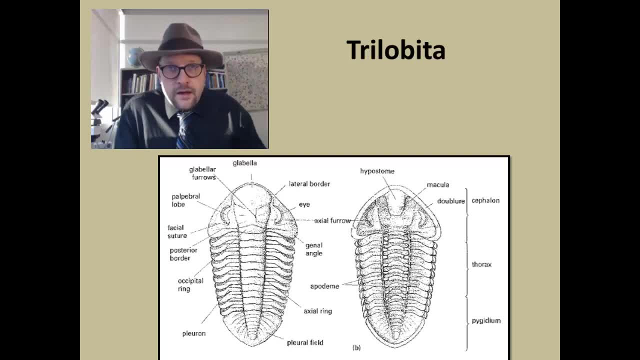 cephalon, with often paired eyes on either side. On the ventral side, if you turn it over, on the bottom of the trilobite is a hypostone, a small plate that's held the mouth and the entrance to the gut tube. 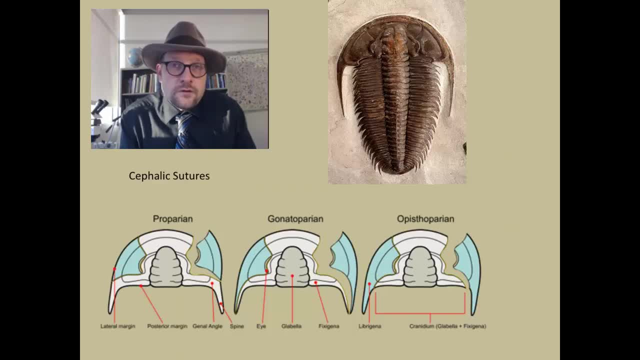 There's a whole bunch of different ways in which paleontologists can describe the anatomy of trilobites in many different conditions. One of the important conditions is the celiac sutures that split the cephalon, and they're used by paleontologists as an important character for diagnosing or identifying various members. 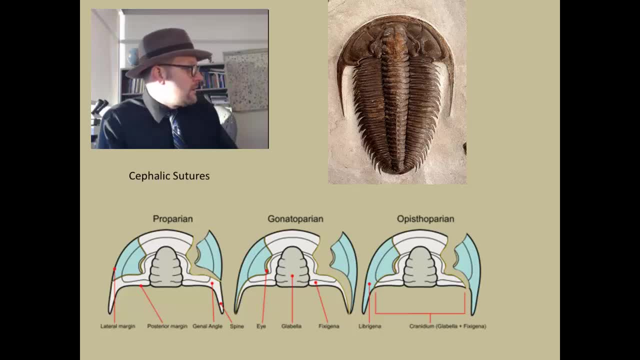 of trilobites. Let's take a look at this trilobite right here. Let's see if we can pair it with the type of celiac sutures that it has. We have the proparion condition, where the side of the lateral margin is not involved. 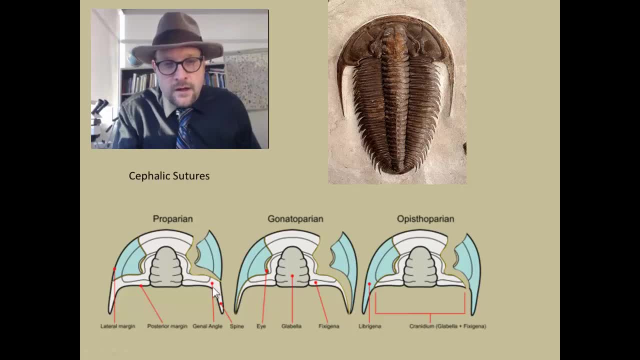 in the spine. The next one we have is the goniotoporion. In this case, the lateral margin here is actually involved in the spine here. Then, finally, we have the goniotoporion, And then finally, we have the goniotoporion. 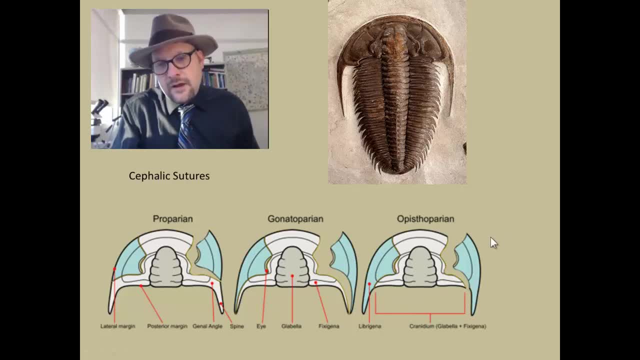 And then, finally, we have the goniotoporion, And then, finally, we have the ospioparion condition, and this condition, the lateral margin here of the cephalon, actually composes the complete spine of the cephalon. So take a look at this fossil. let's see which one it is a member of. 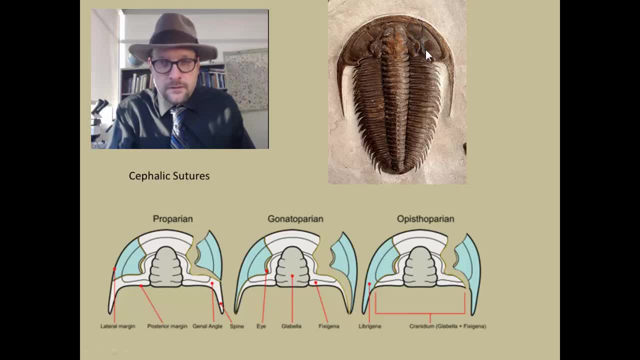 So we can see there's the suture coming down through here. it comes down over here. oh, you know what looks like. it's the last one. Hopefully you agree. so it's the last one there, Alright, so let's look at another character. 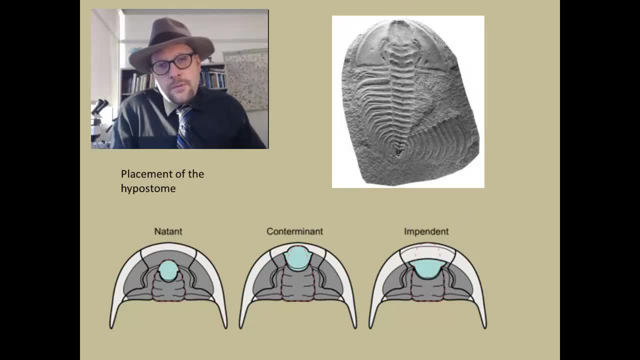 And this is the placement of the hypostome on the ventral surface. so this is on the bottom surface of the trilobite. We got the nadolent condition. this is where the hypostome does not contact the margin of the cephalon. there 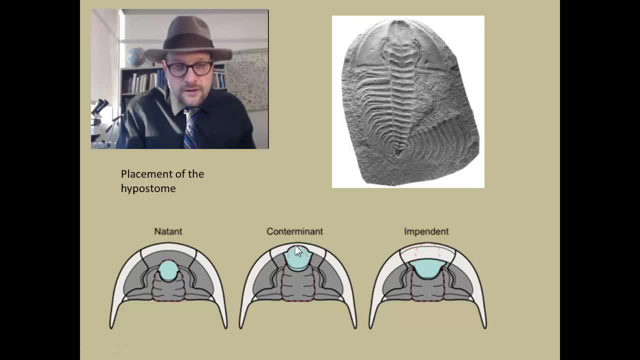 We have the countermentent condition in which it does contact the lateral margin. And then we got the impedient in which the lateral margin is outgrown: it contacts it, but it is greatly expanded. So let's take a look at this fossil trilobite and try to determine which one of these three 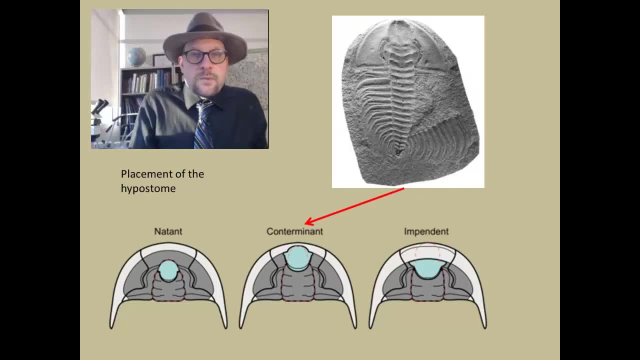 conditions it has. Alright, yes, it is the middle condition here. so it's the countermentent. you can see that the hypostome extends all the way to the margin there and the margin is not really thickened. Now, the anatomy of trilobites is a little bizarre. 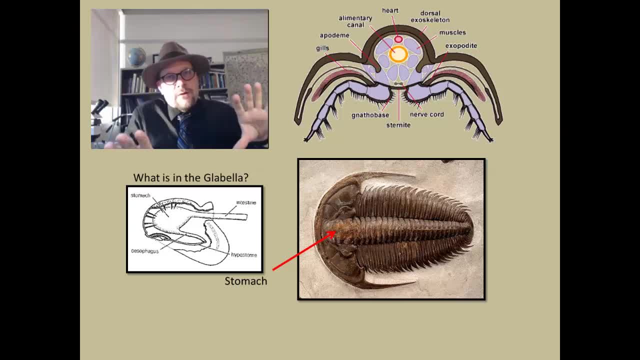 So that bumpy thing on the front of the head is not the nose, but it's the stomach and that's called the gababelle. It actually holds an expansion of the gut tube, so it holds a stomach and then it has the mouth opening on the ventral side of the trilobite. 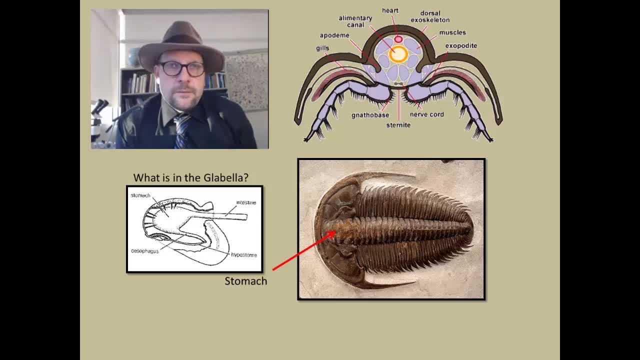 The other weird thing about the anatomy of trilobites is that each of the limbs are paired with a gill so that as it moves along the ocean floor, the gills would get a fresh supply of oxygenated waters from the movement of those limbs. 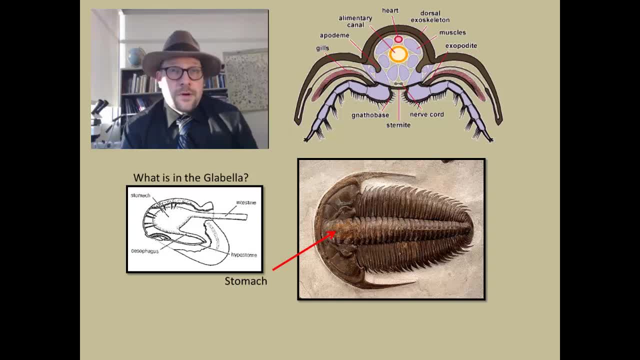 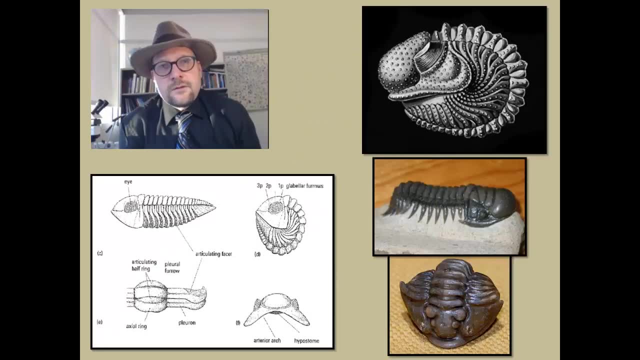 This is similar to what many arthropods do In land. many arthropods develop book lungs that are underneath their porous exoskeletons. Now the exoskeleton of trilobites is made out of low magnesium calcite, which is a hard. 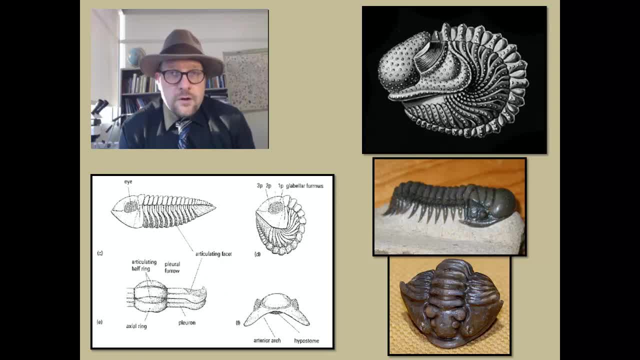 material that can be used for protection, and trilobites can coil up into balls for defense. In fact, many fossils have been found with trilobites in these coiled defensive positions. Because the exoskeleton of trilobites is made out of low magnesium calcite, trilobites can 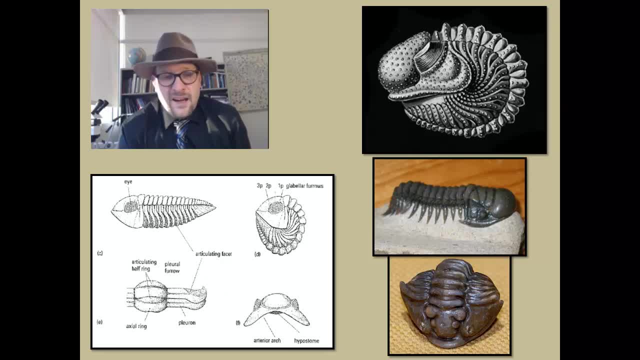 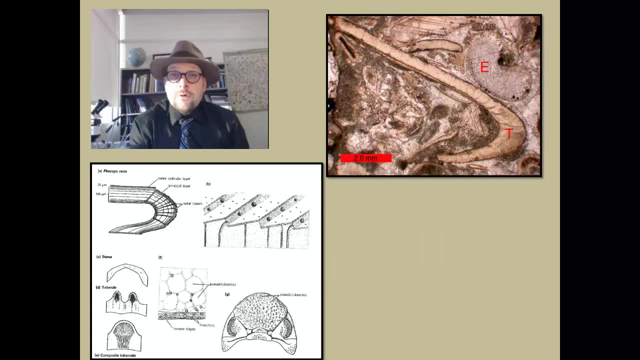 be used for protection. The exoskeleton of trilobites is made out of calcium calcite, and it readily preserves in the fossil record as well. The exoskeleton or cuticle of trilobites is composed of two layers: a relatively thin 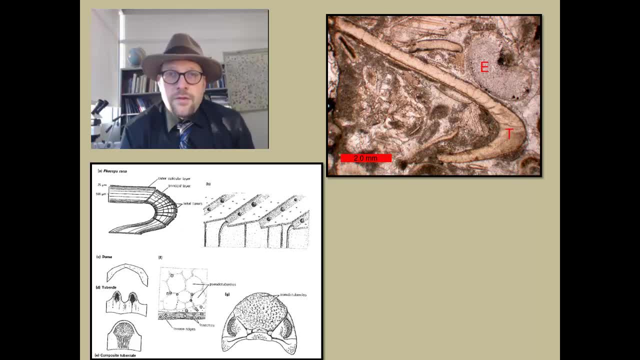 outer layer with very large calcium calcite crystals and a much thicker inner layer of tiny calcium calcite crystals. This inner layer is formed in small lamellar sheets, which provide some flexibility. There are oftentimes little pores Or canals that run through the exoskeleton, and these likely serve for small hairs or 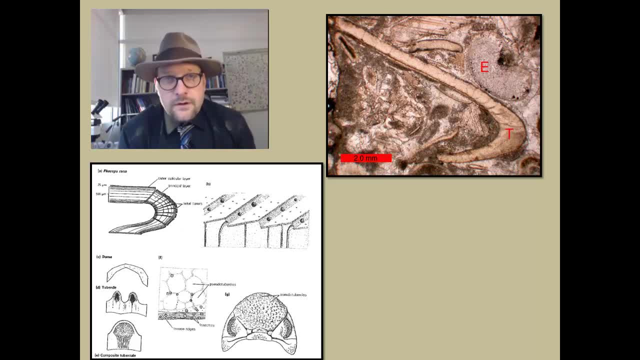 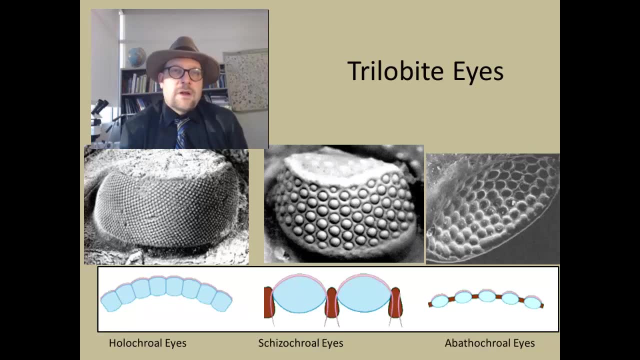 setia for sensing the environment outside the exoskeleton. Perhaps the most remarkable adaptation of trilobites is the development of eyes. It is the most ancient of the visual systems known. Trilobites have compound eyes, like modern crustaceans and insects. 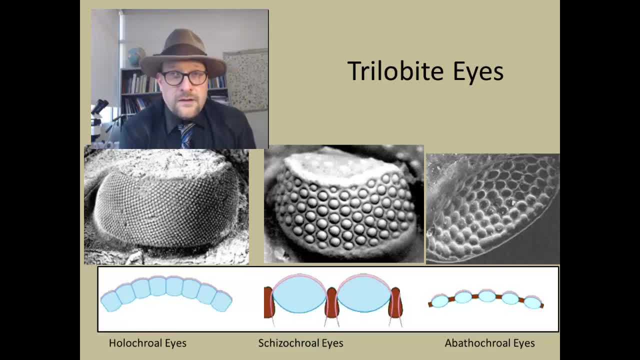 However, since their exoskeleton is composed of calcium calcite, which has a high diffraction of light, The crystal lenses that compose the eye need to be arranged just right to prevent any sort of distortion of the images. Most trilobites have eyes that are what we call the holochoreal condition. 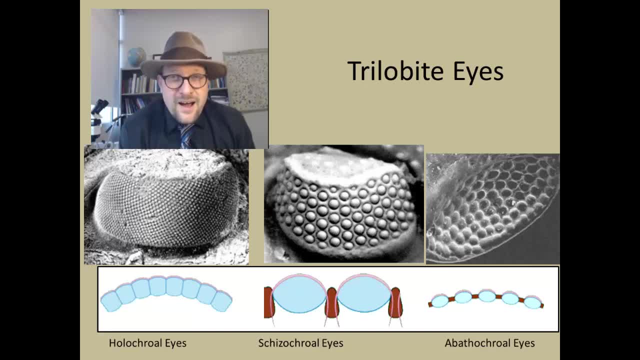 This is where the lenses in each eye are in contact with each other, and then the entire lens is covered by a corneal membrane. A more complex eye is found in the Phychiopoean trilobites. This is called the sclerochoreal eye. 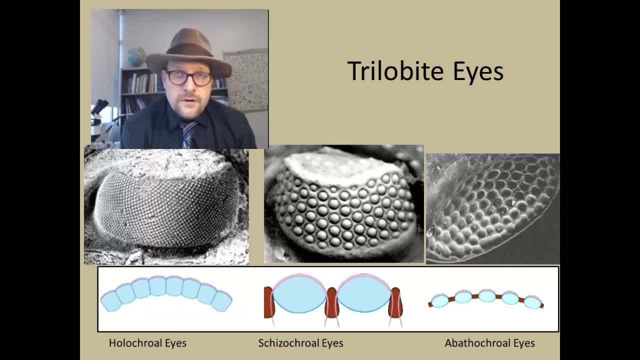 These trilobites differ in having an interstellar material called sclera between the lenses. The lenses are really broad and really big. The light in these trilobites is more complexly focused and it provided prior visual senses even during periods of molting, when other trilobites would be blind during the process. 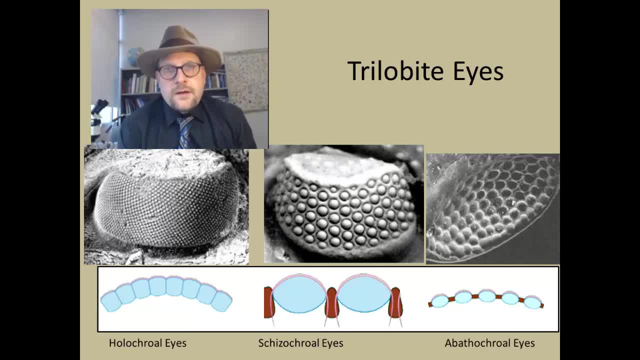 of shedding. The last type of eye of trilobites are the abathochoreal eyes. They are found in the order Agnothista, which includes many blind trilobites, and as such it probably represents a reduced or vestigial sclerochoreal condition. so they are on the 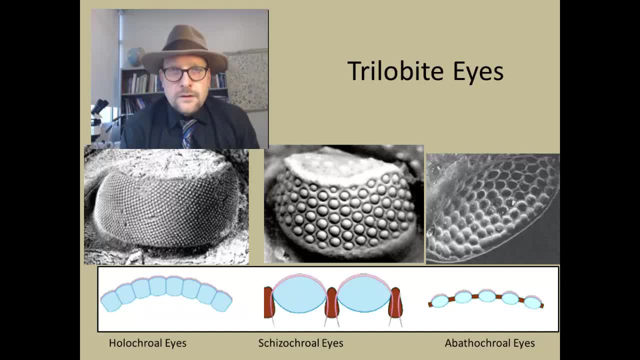 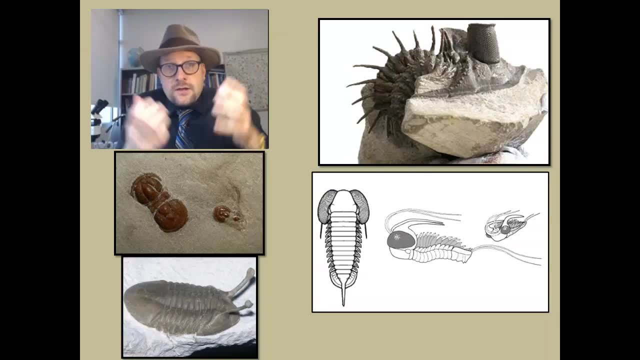 way of losing their eyes and becoming blind. There is a huge variety of trilobite eyes represented in the Phococoreal eye. Some had giant eyes and likely used those that were nectonic or swimming along. Others had very broad eyes, great for low light conditions on the bottoms of the ocean. 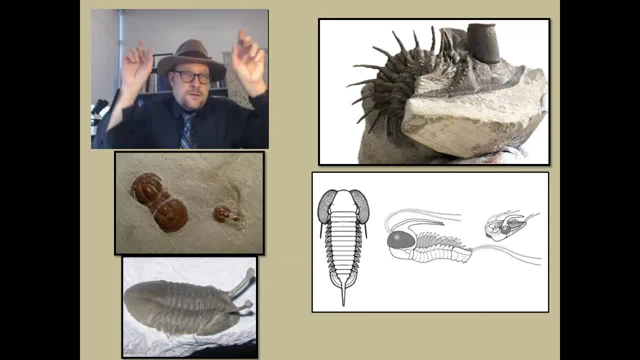 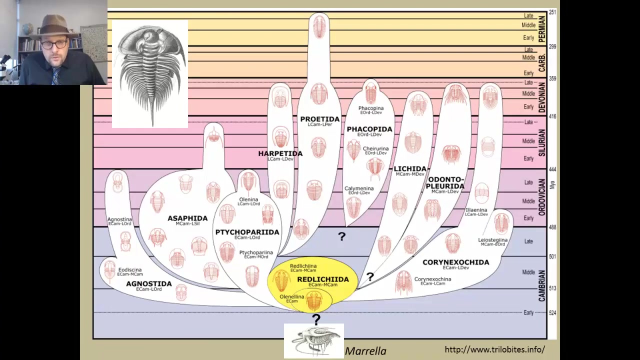 Others had eyes on long stalks so they may raise those eyes above muddy substrate. And then there are many examples of trilobites that go blind, lose their eyes and swim around completely blind. I thought I would go through and discuss the various groups of trilobites and give you 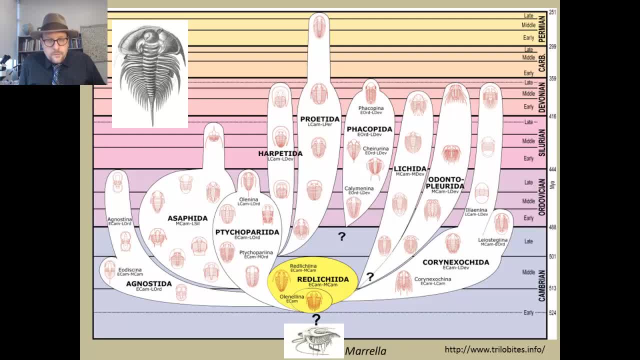 some pictures of some of the diversity of these various groups. Trilobites originate during the early Cambrian, probably from something like Maraelia, and the first group we get to is the Redlynchia. The next group is the Redlynchia. 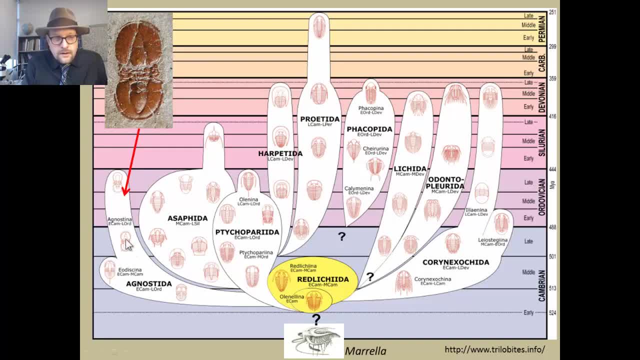 The second group is the Anthnozoidae. These include many of the blind trilobites And they are kind of peculiar in the fact that they have the double feature. These were believed to be swimmers swimming around in the water and using the two ends. 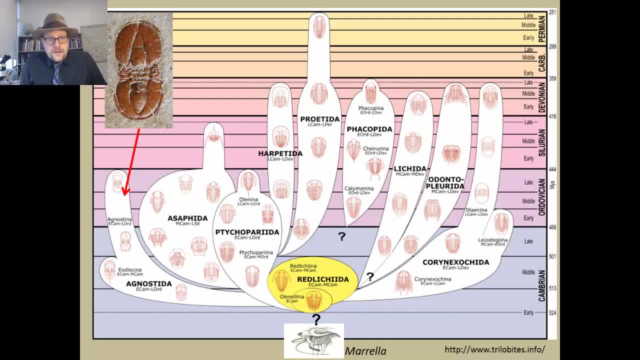 the very enlarged patygeum to swim around and gather food in very low light conditions. The next group is the Aspidifloridae. These include groups that go from the Middle Cambrian up to the Late Silurian. The Aspidifloridae are the most common trilobites. 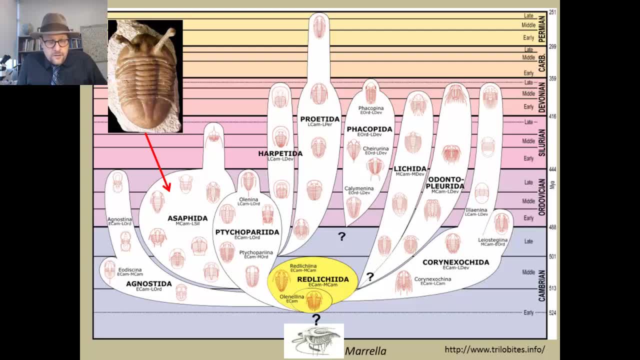 They are the most common trilobites. The Aspidifloridae are the most common trilobites. They include the members that have the long stocked eyes, The Picroparidae. This is the next group. 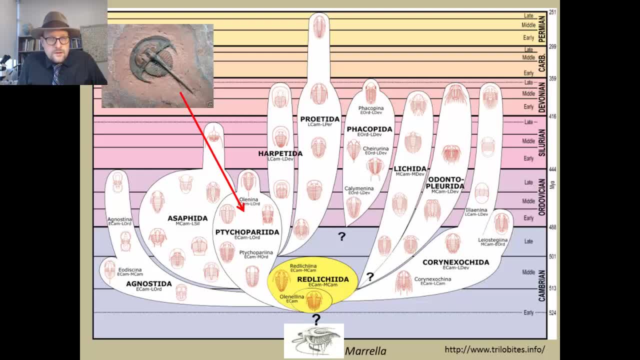 These are known also from the Middle Cambrian into the Ordovician. They include these groups that have very enlarged cephala and sort of short little bodies or pleural lobes. Another group that has very large cephala are the Harpipaedid. 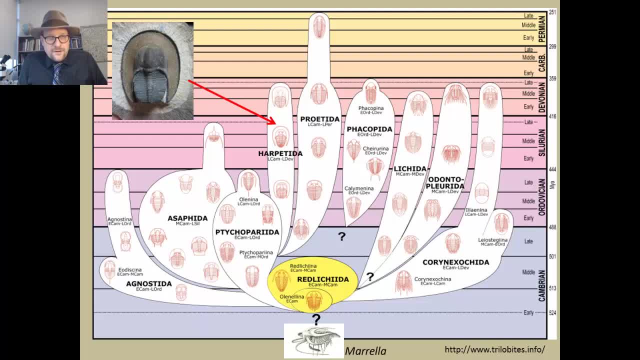 These guys have these very ring-like huge giant cephalons that extend with these very long stalks. They have very long spines. They extend almost to the entire length of their bodies, which is pretty impressive. The next group is the longest-lived group. 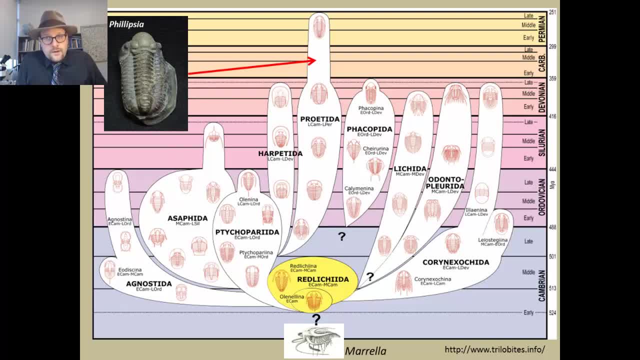 This is the only group to have made it through into the Carboniferous and the Permian. So you can see that at the end of the Devonian many of these groups start to go out and start to disappear. This includes the very common Philipsia. 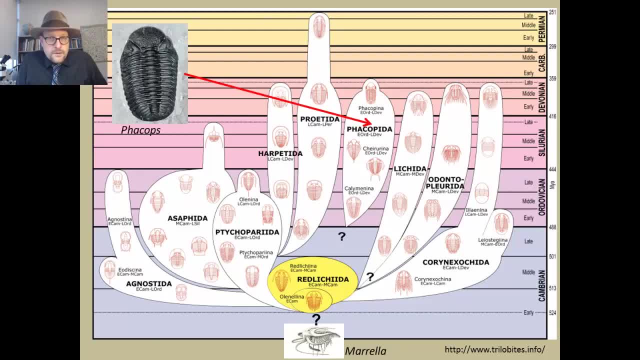 Probably the most famous and more common of the trilobites is the Phakops or the Phakiopidae Phakiopidae. These are the ones with the very complex eyes. These guys can actually get pretty big too. 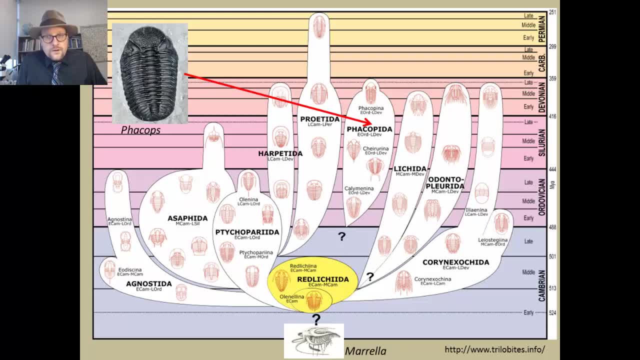 I've seen some large ones in collections and they're known from the Ordovician to the Devonian. We then have the Lachodeids. These go back into the late Cambrian. They're characterized by having sort of- I don't know, like a broomstick sort of legs. 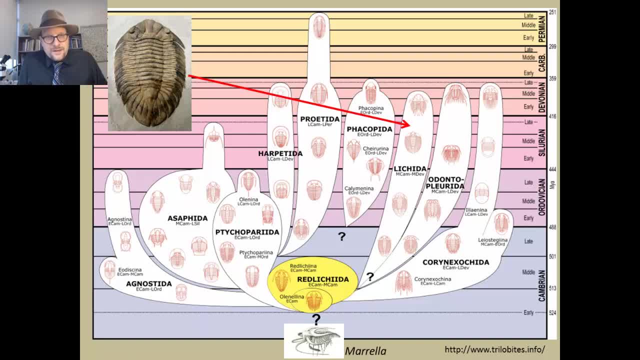 segments that come out and sort of sweep out, which are very unique. The Odontopluraidae- This is a group that includes the very spiny. This is a group that includes the very spiny Trilobites. These are often very popular with collectors because they have these very long, delicate. 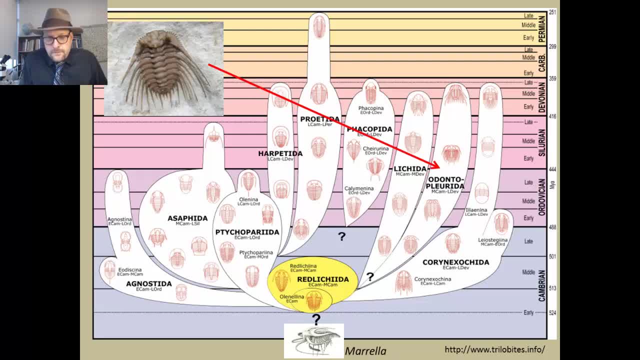 spines that often preserve in the fossil record. And then we have the Chloronexaceae. These are a group of trilobites. Some of them have spines, but many of them forego those later on, And they extend all the way up into the Devonian. 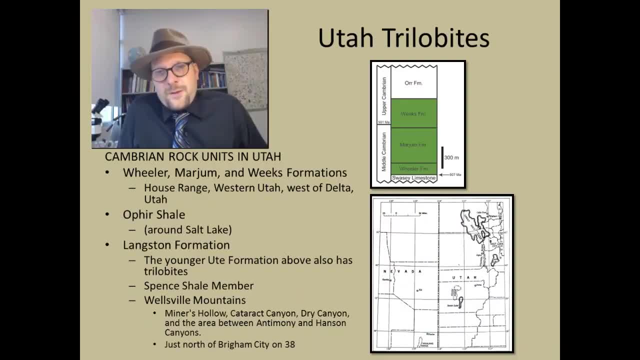 All right. So you might be wondering, like, where to go to find some trilobites. So I was going to talk a little bit about Utah's record of trilobites very briefly. So Utah has a fabulous record of trilobites. 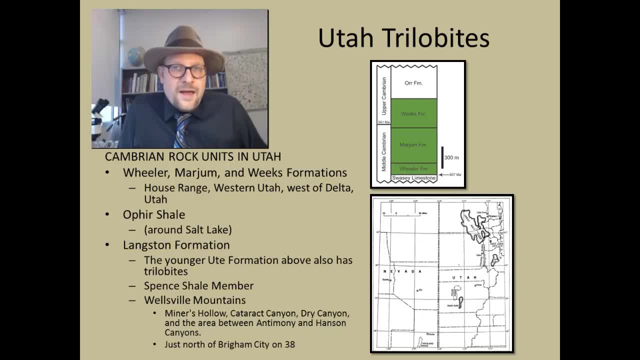 There's sort of two states that have really good trilobites, That's New York and Utah. Most of New York's trilobites are Devonian And most of Utah's trilobites are all Cambrian, So there's a great record of Cambrian trilobites here in Utah. 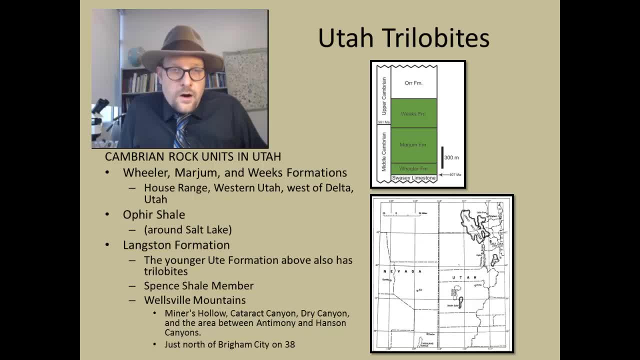 The most common formations in which trilobites are found are the Wheeler, Marjum and Weeks formations, And these are exposed in the house range which is in the west, And these are exposed in the house range which is in the west. 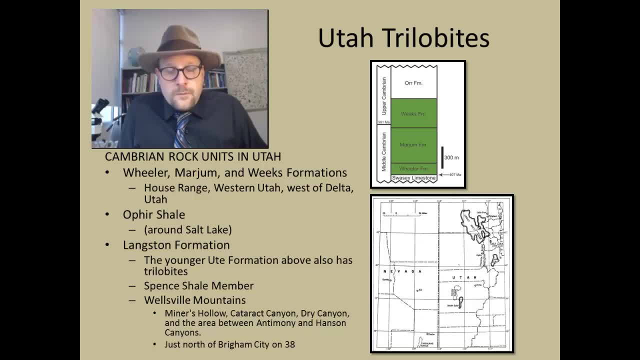 So these are exposed in the house range which is in the west And in the western part of Utah. out in the Great Basin there are many sites west of Delta Utah where you can go and collect And there's some places where you can pay the landowners to go on to their property. 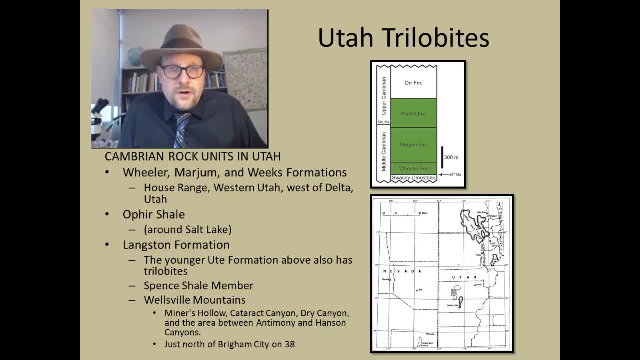 and collect in quarries and they sort of guarantee that you'll find trilobites there. If you're closer around Salt Lake, the Ophrah Shale does produce some trilobites. Another place where trilobites have been documented is the Langston Formation and the Younger. 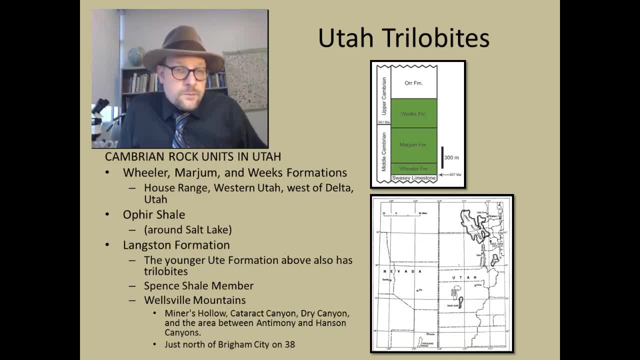 Ute Formation that also has trilobites. So these are some of the places you can go to find trilobites. Trilobites, as well as the Spence Shale member. Many of these sites are located along the Wellsville Mountains, just sort of north of. 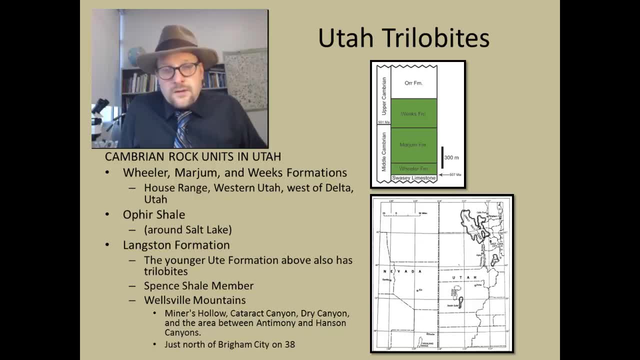 Brigham City, Utah, in western Utah. So many of the sites in western Utah contain trilobites. In eastern Utah there's fewer trilobites found. That's because most of the Cambrian formations are sandstones and don't produce the nice. 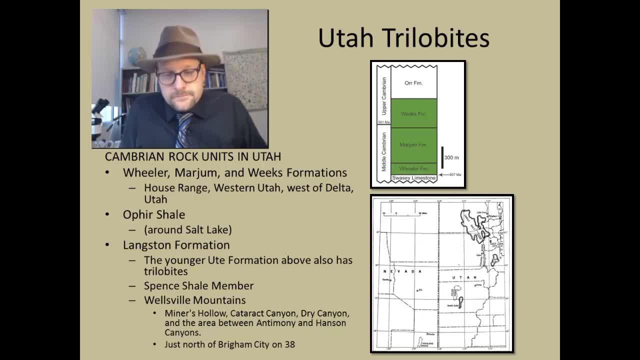 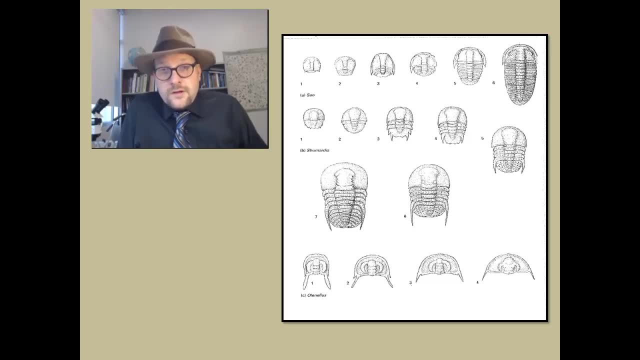 shales that really do a great job of preserving trilobites. One thing just to remind you about trilobites is that they do shed So many times. when you do collect trilobites and are trying to identify them, you need. 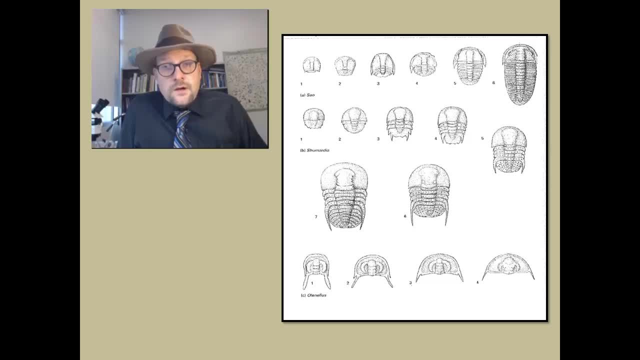 to be aware that there are an ontological series of sheds and so many times trilobites that look very different might be the same species and you're just seeing younger individuals. So be aware of that whenever you're out collecting and trying to identify trilobites. 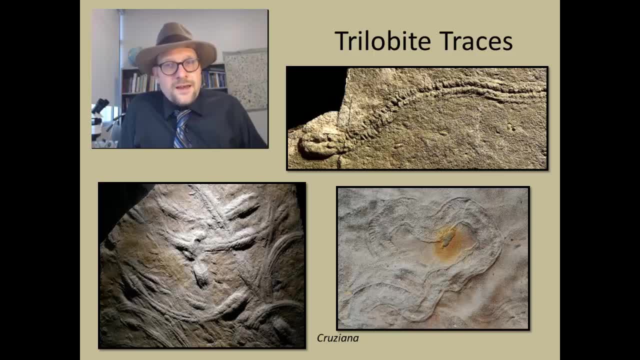 One last thing before I sign off about trilobites is that they leave behind wonderful traces in the fossil record, and many of these traces have been documented throughout the Paleozoic. This is a trace fossil that's very characteristic and it's called Cruzana. 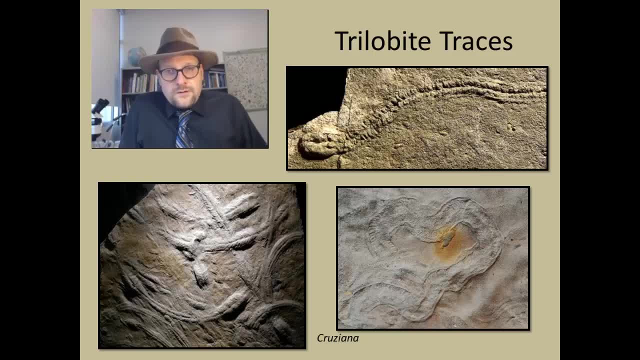 Cruzana can be recognized because you see all of those little individual legs digging around, scuttling around in the sediment and then oftentimes you'll get a rest trace where the little trilobite kind of nestles down into the mud. 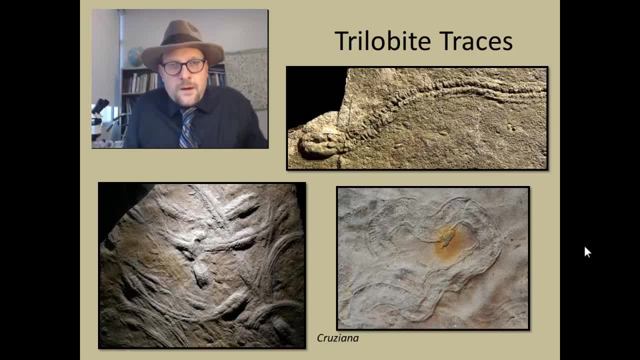 Then it scuttles up and scuttles along, so you see lots of those little legs moving, making lots of little footprints along as they scuttle around, and then oftentimes you'll find like a rest places where they stopped and rested before they scuttle on. and oftentimes